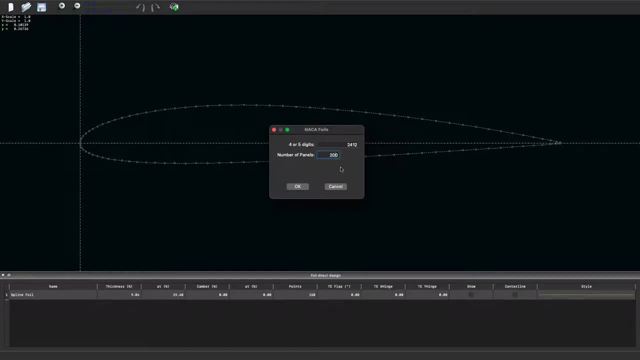 do 200 panels. You know you can see 200 panels. All right, So that's 2412.. Click OK. What I'm going to do is also make sure that I can see the airfoil clearly, because you know you have a. 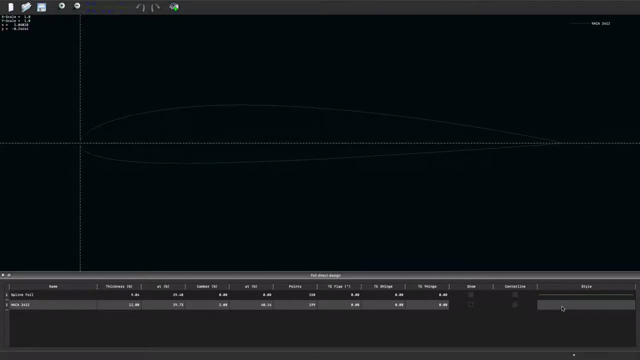 black background. Chances are you're probably not going to be able to see it, you know, in the video. So what I'm going to do is actually click this like style right here. So I'm going to go to color and I'm going to make it a little thicker And then essentially, I'm going to add, like, some markers. 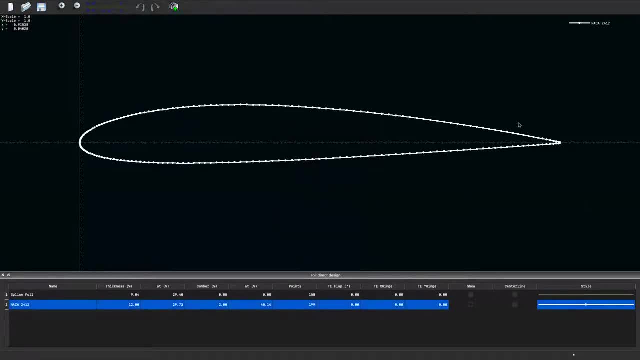 So now you can actually see the profile very clearly. right, It's a 2412 airfoil that we're going to work with And, yeah, you know it's all set. So you know, this is the airfoil that we're. 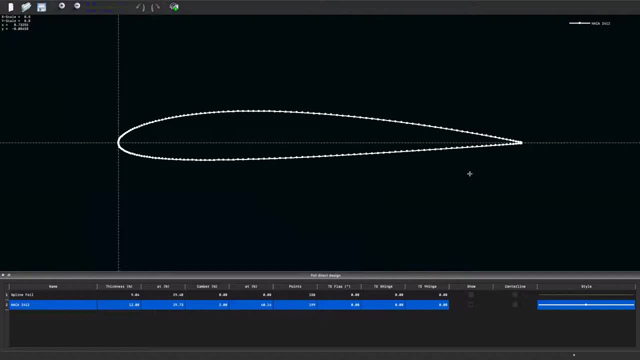 going to use Right? So now we have an airfoil, Let's go to the XFOIL direct analysis, But before to include them as well, you know, for example, you know I can load another airfoil in here. 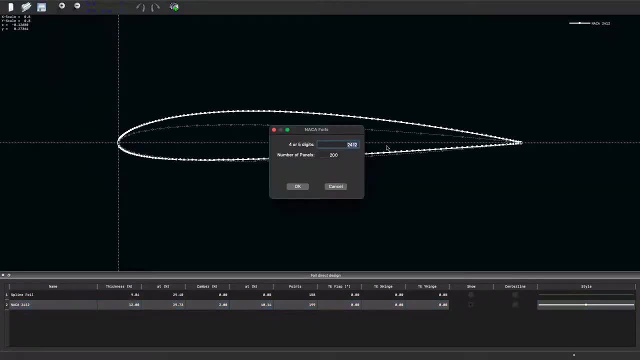 Right, Go to do NERCA foils And I'm going to do, instead of 2412, let's do like 0012.. Right, 200.. OK, That's 0012.. Now I'm still going to change the color a little bit, maybe add like a fluorescent. 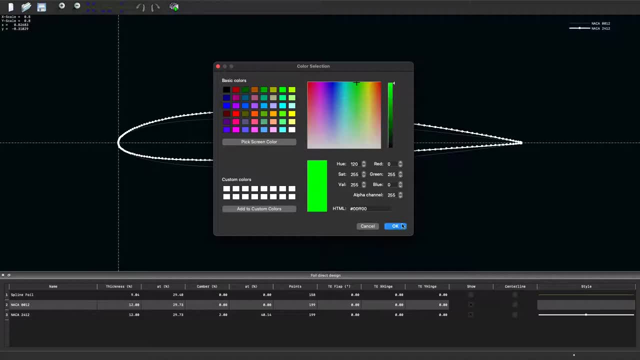 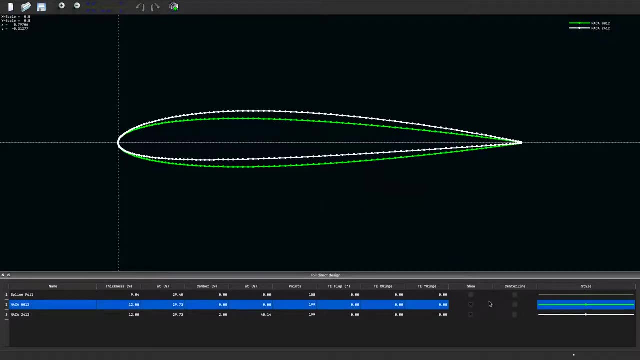 blue or green. Right, So, right here, so that I can see better, And then again change the width, add some pointers. OK, So now you can see the 0012 as well, Right? So in this stage, load all the airfoils that you. 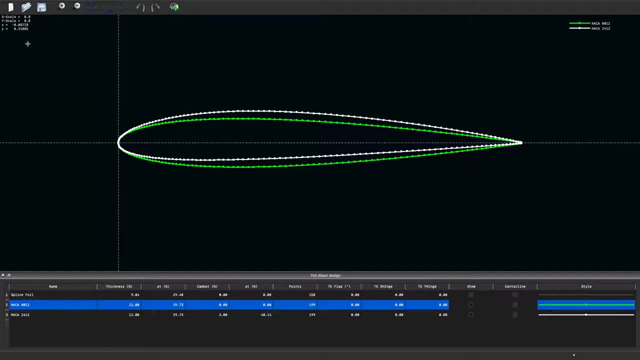 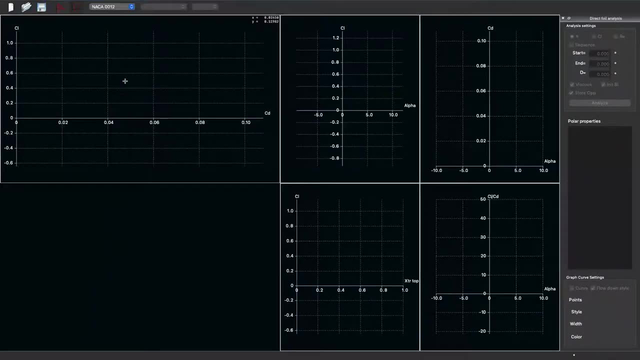 want to use, because this will pop up later in the software. OK, So now let's go to FOIL and let's run- sorry. let's go to file and do the direct FOIL analysis: Right, This window will pop up. The first thing we need to do is define an analysis Right, Because before we analyze the 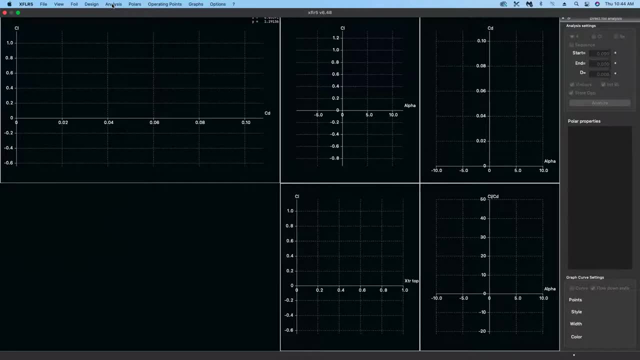 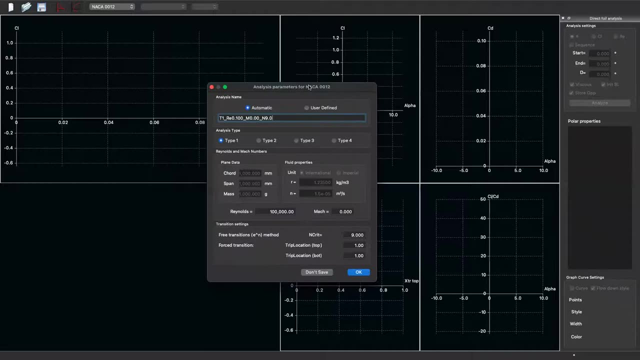 wing, let's make sure the airfoils are working properly and you know showing what you expect to show. All right, So let's go to analysis. do the defining analysis. This window will essentially pop up Right Now. I'm going to add, you know, whatever the Reynolds number that you want you can simulate. 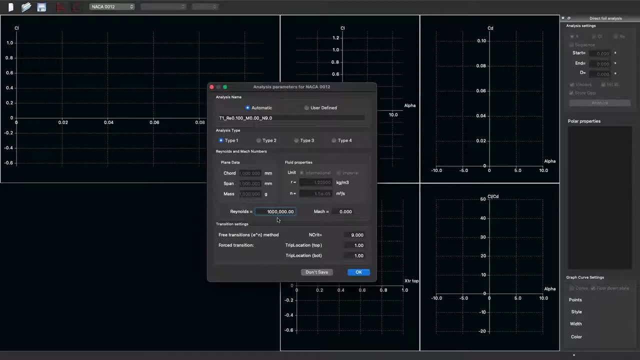 it. But I'm going to put like about a 10 million Reynolds number here, Right, But you know I would. I would urge you guys to calculate the actual flight Reynolds number that you want to simulate and then you know, click OK, Right. So now. 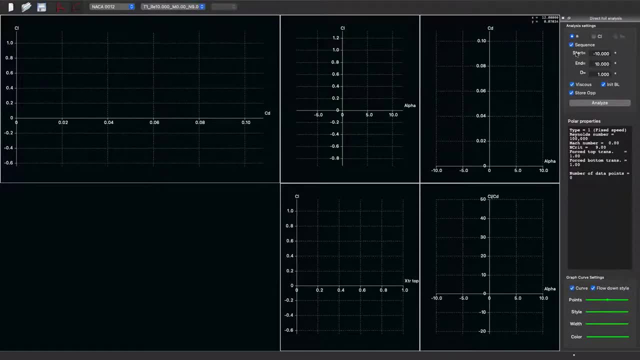 You know, you can see that this tab- direct FOIL analysis tab is, you know- is popped up. Now you have to choose the airfoil, Right? Do you want 2412 or 0012? Right, So the analysis tab is actually active for 0012, but not for 2412. Right, So I can go here and, you know, first run the 0012 and then come back and run the 2412 as well, Right. 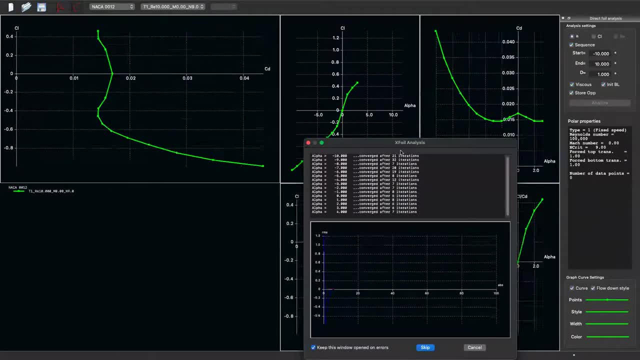 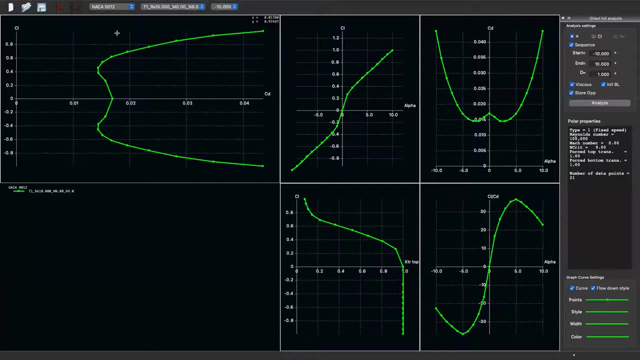 So, define the analysis. You know I'm going to click analyze. You can see that it's plotting a nice profile right here, Right 0012.. Now what I can do is, you know, go here, change to 2412,, go back to analysis. you know, define an analysis. 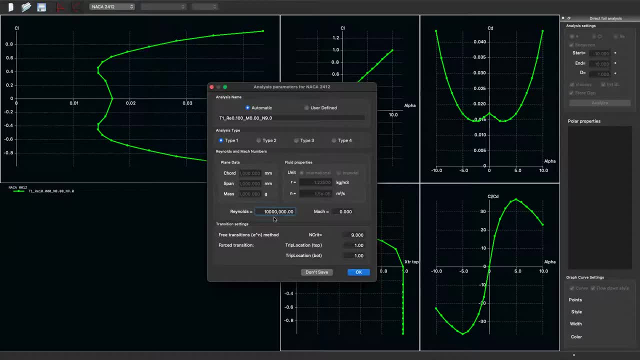 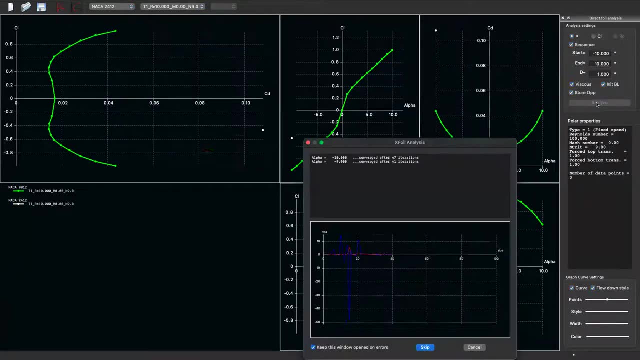 Again, I'm going to simulate this and then in the Reynolds number, 10 million as well. OK, Right, So now I'm going to go through the same do the analysis. Now you can actually see that two airfoils performance curves- Right. 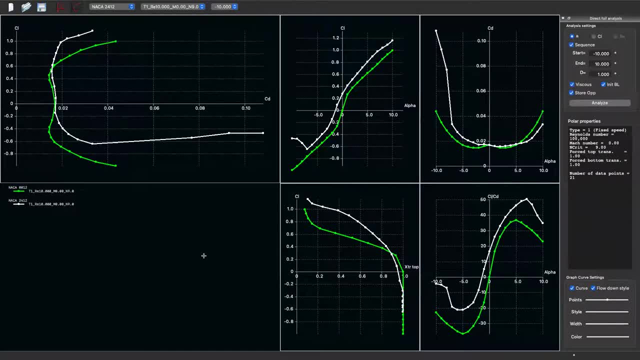 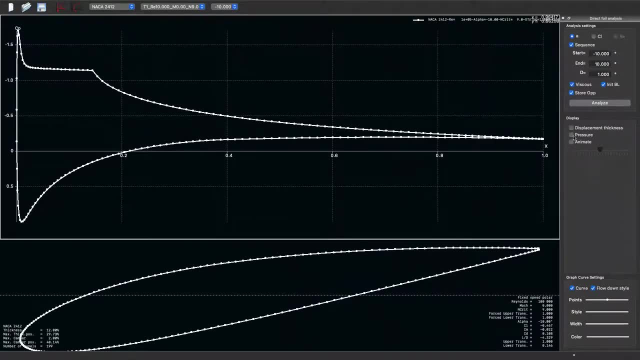 CDL versus alpha CD versus alpha, Right, Right here, Which is again pretty cool, You know, and if you actually go here you can actually see the CP distribution Right. You can also see the pressure distribution on the airfoil. 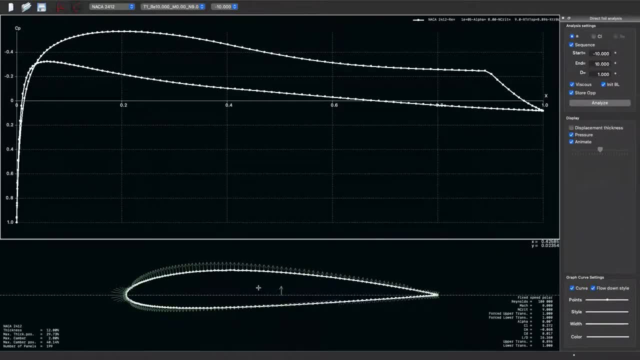 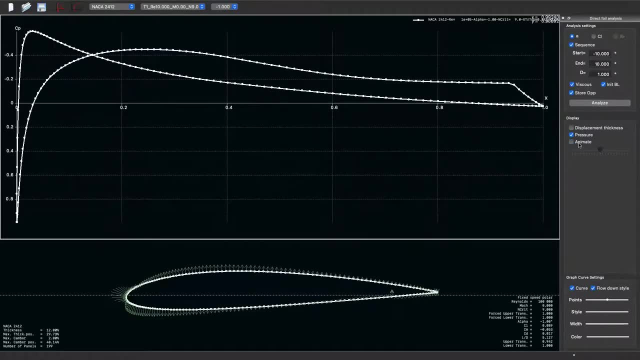 And if you click animate, you know you can go through the different angles of attack and show how the pressure is distributed around the airfoil, Right, So it's. it's again all cool. You can do this for 0012 as well, Right. 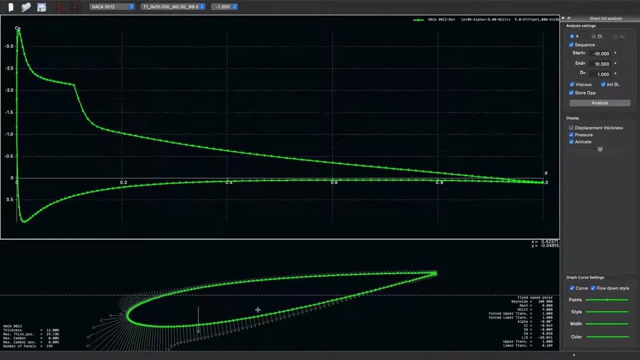 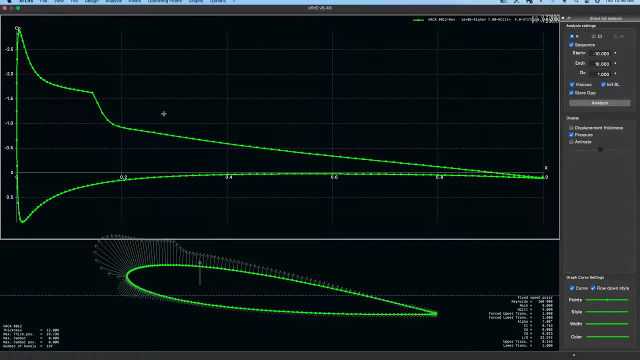 You can click animate and then it'll Go through and show you the CP distribution. All right. So we know, we now know that the airfoil actually works Right, Showing what we expect to see. There's no problems in this stage. 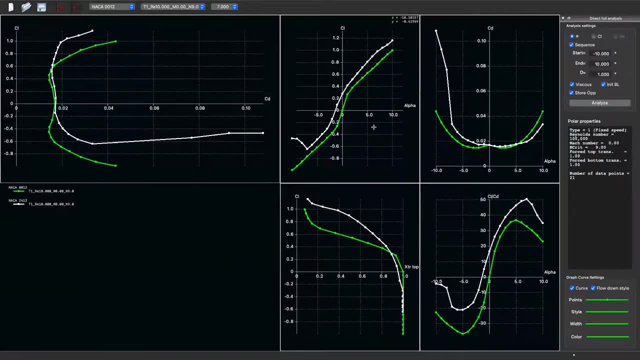 So once you know that there is no problem in XFLR5 simulating the CL versus alpha of all of these, you know performance curves, you know for an airfoil, you know that, you know you can proceed to a wing analysis. 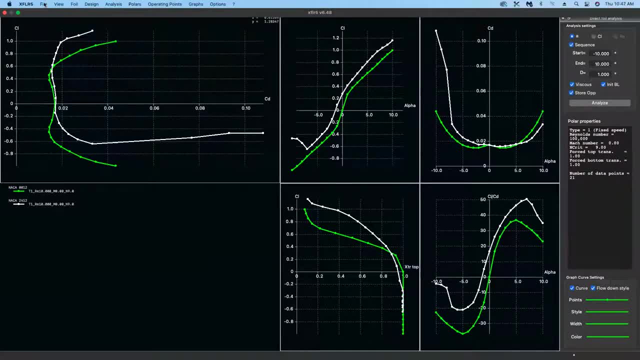 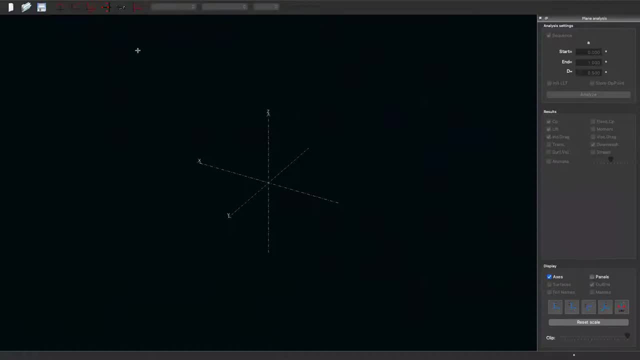 Right Now, let's do that. You know, let's go to a file And now let's go to the wing and plane design. All right, So the wing and plane design. you know, sometimes you know you will have multiple windows open up. You know you have three. you know you have like six different tabs here, Right, 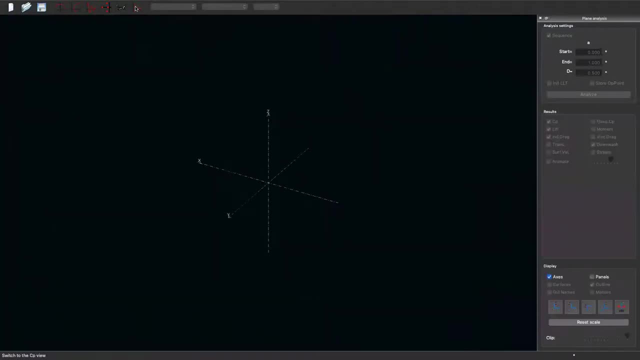 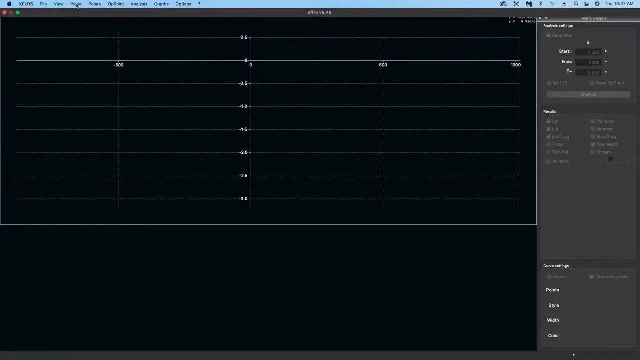 So these are the. this is where you will actually see all the data. You know, we'll take it step by step. So before we even do the analysis, we have to define a plane or we have to create an airplane- Right. 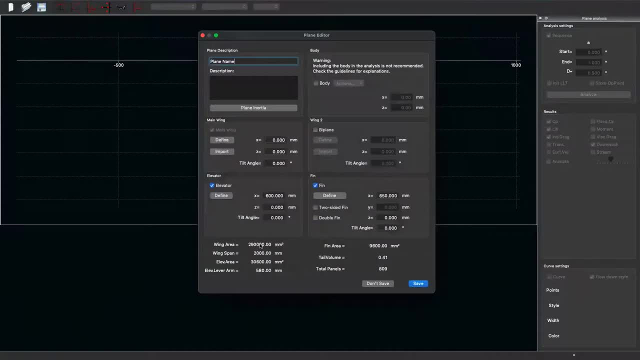 So it's going to plane And do a, define a new plane. All right Now in XFLR5, you can have an elevator, fin fuselage, the wing, etc. But here we are only interested in the wing. 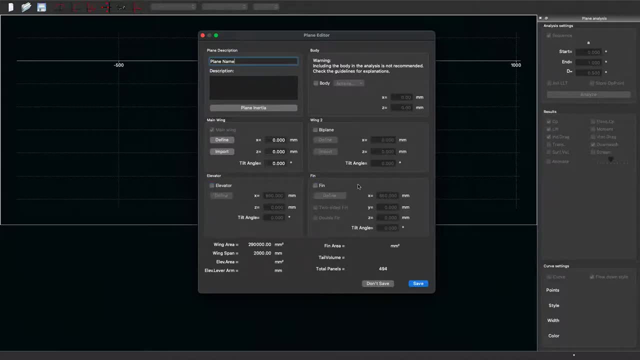 Right, So let's, You know, let's uncheck the elevator and the fin, Let's have the main wing alone. Now I'm going to label my airplane as like Panel D, You know, wing Right, So Panel D wing. 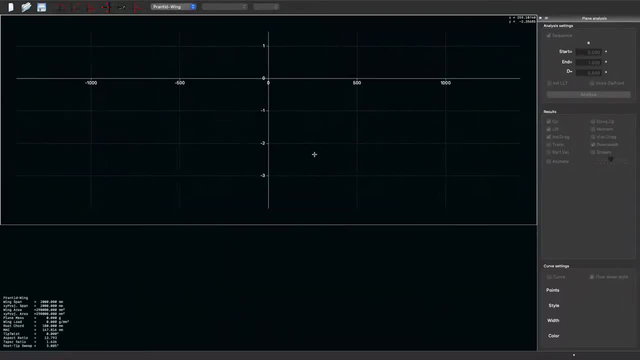 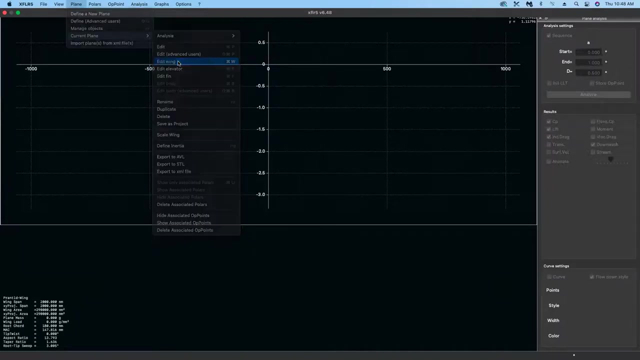 Click Save. All right, So now I have my. I defined the plane, but I haven't actually changed anything in the wing right. So, in order to you know, design the wing itself, let's go to plane, go to current plane and then do edit wing. 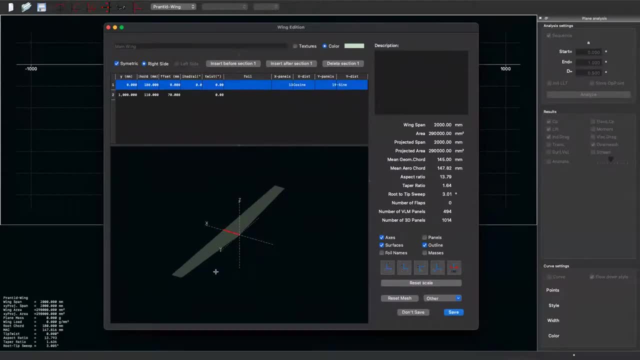 So when you press edit wing, this window will pop up right. This is where you can actually design your wing any way you want, all right. So again, you can add multiple sections, and you can add as many sections as you want. you know, design your wing piece by piece. Now we only have two. 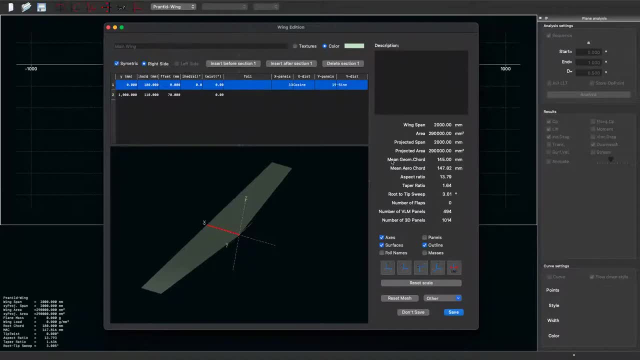 sections. The first section right here which is highlighted is in the root, and then the second section is actually in the tip. all, right, So you can see that red dots popping up right, or red lines. So that's the two panels, right? That's what you're defining here. 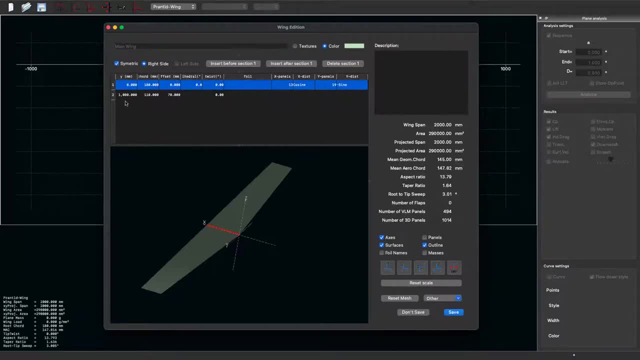 So the root code is at 0, 0,. right, Now I can set my y, you know, to be like, you know, 1000.. 1000 millimeters, right, You know that's. you know you can design your wing to any shape. 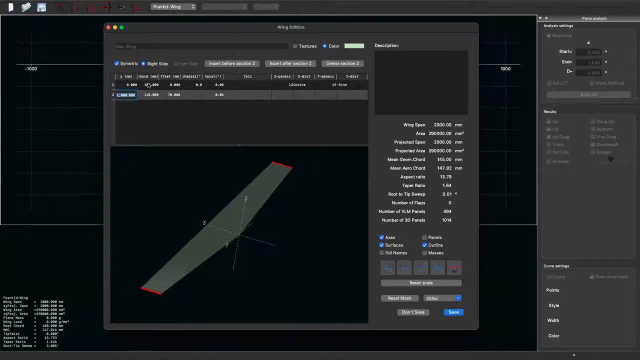 any length you want. So I'm just going to leave it as such, like 1000 millimeters, and I'm going to change my code at the root to have the same code as the. you know the tip. So I have 100,, 100, right, So I have like 100,, you know, or you can do like even 200,. 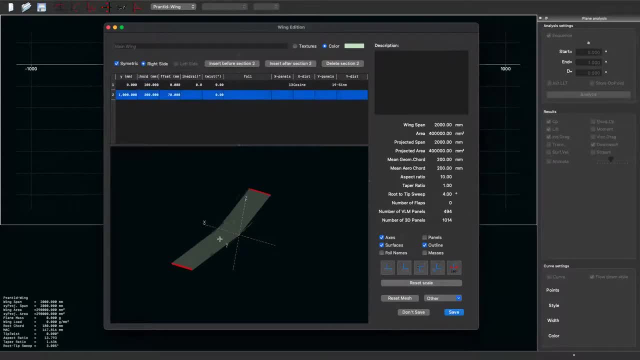 right. You can actually see that by changing these values you're essentially changing. you know the length of the wing, So I'm just going to leave it as such. like 1000 millimeters, right. So now you know you have the same code and root and the tip, but you have a little bit. 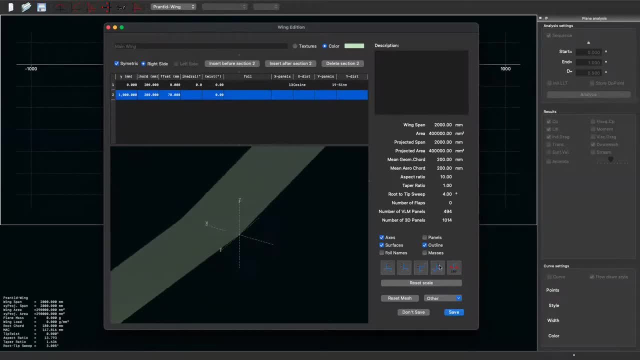 of offset, which actually puts sweep on your airplane- Say: if you don't want your sweep, then just come here and set it equal to zero. right Now you have a rectangular wing right here, right? If you want, you can add a dihedral, But you know, for now let's just keep it at zero. 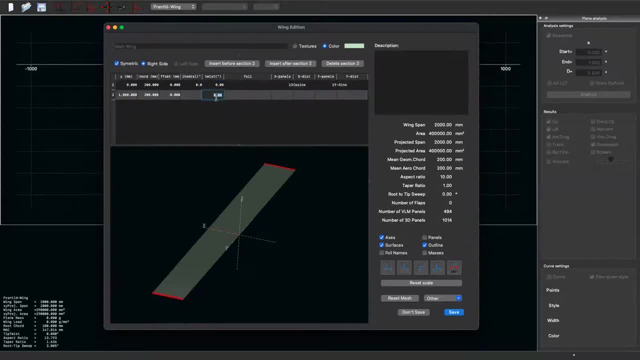 If you want, you can add a twist And again, for now we'll just keep it. here's where we select the airfoil. Now what I'm going to do is you can see the two airfoils that we simulated. you know the previous step popping up here, right? So I'm going to put my 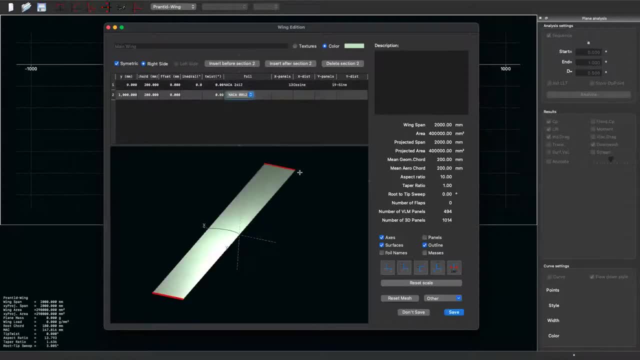 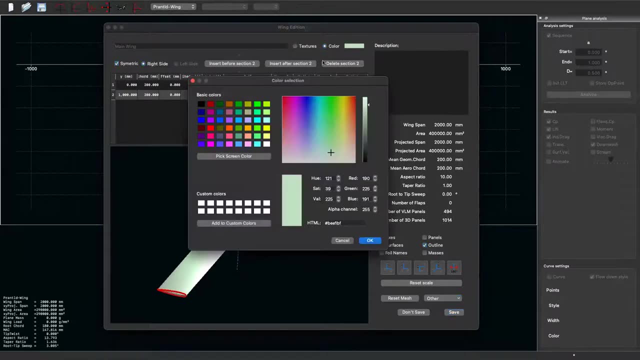 root code as 2412, and I'm going to put my tip code as 0012,. all right, Now I can change my color. you know, of the wing. you know, if you press color right here, you can actually see. 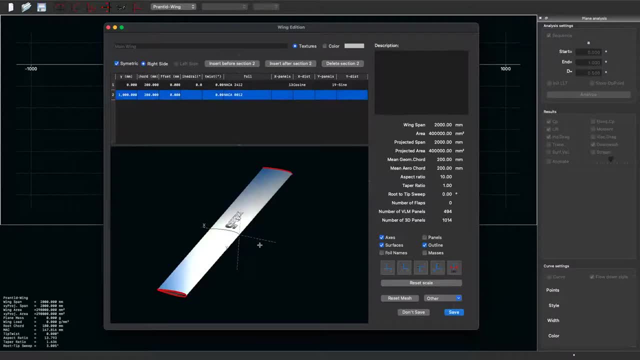 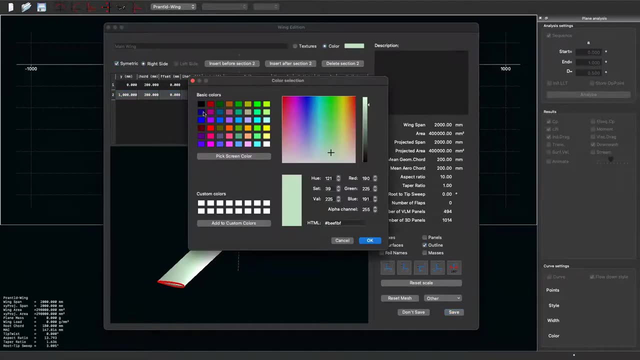 you can even select textures. as you can see, you know you have a textured wing right, So again, you can change the appearance to anything you want. So what I'm going to do is I'm going to put a dark color here so that you can see some of the things, some of the properties, pretty clearly. 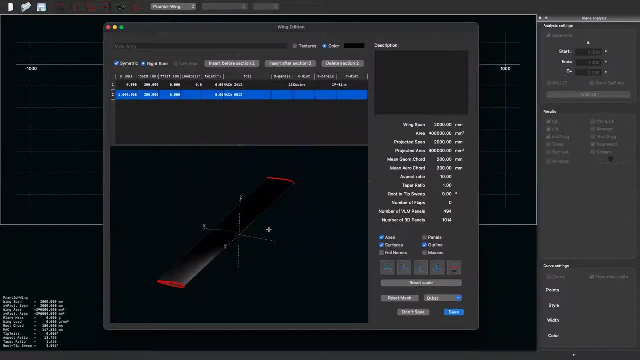 So I'm going to put black. you know black. you know you can not see it very well, But what I'm going to do is if I actually click this panels icon, you know, right here in a panels icon now, you can actually see the wing pretty clearly, right. So this is essentially the wing that we 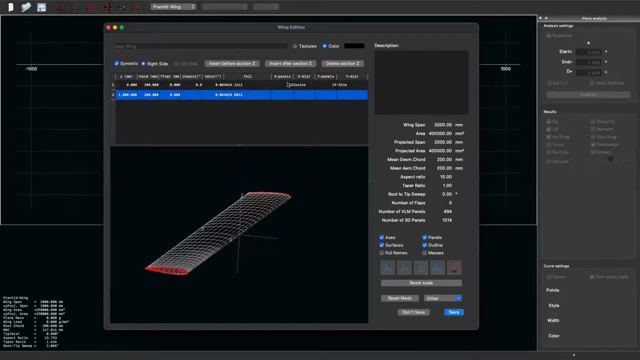 just simulated. right Now you can see that the number of you can control the number of panels by using this. like these, like panels right Now, you can change the number but make you know if you have a large number of panels. it will take a lot of computational time. 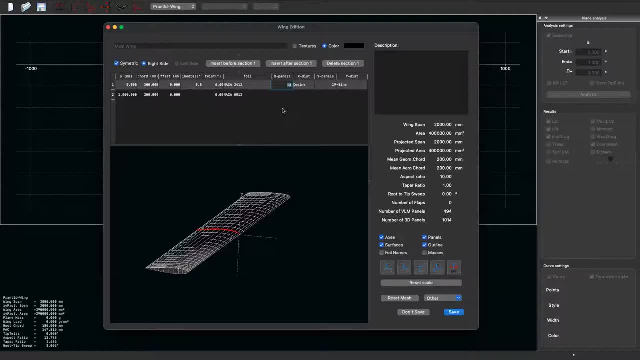 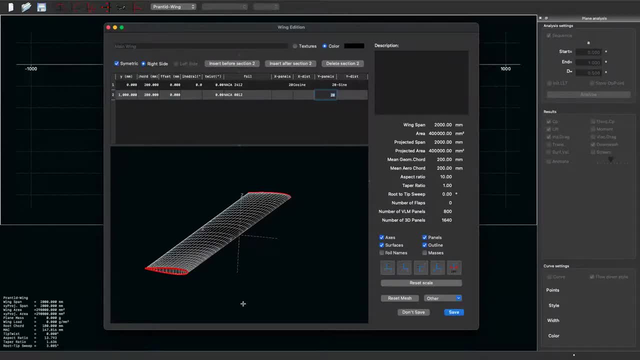 I would, you know, just keep it as sine and cosine, as you know, whatever it is, Because you know, if you put uniform distribution, what happens is that your leading edge and trailing edge may not be, may not be resolved clearly. all right, So you can see the wing right here, right, You know? 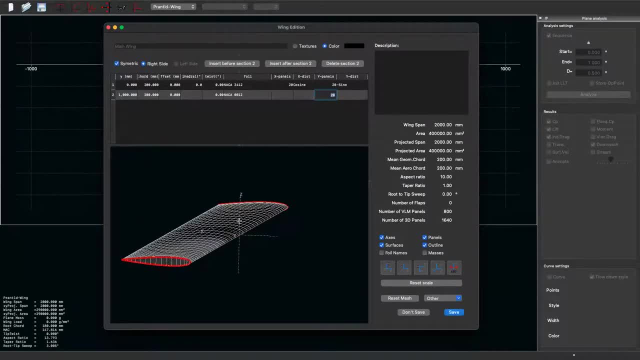 it's a pretty, pretty straightforward wing, rectangular wing. nothing too complicated about this, except you know you have a. you have two different airfoils in the root and the tip right. So again the wing, the XFLR5. 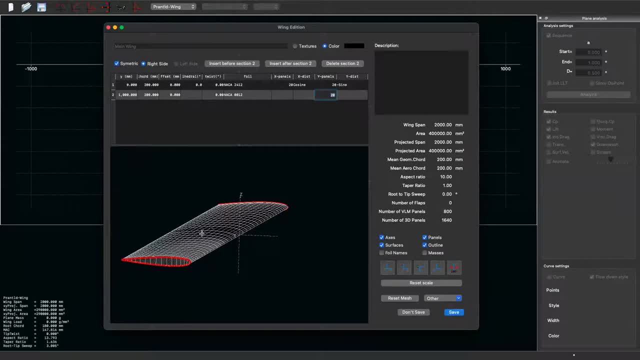 actually, like, lost the connection. So, therefore, you know, if you actually take a profile in between the root and the tip, you know you're going to get a blend of 2412 and 0012, right, It's not like you have a 2412 at the root and 0012 at the tip alone. You know you have this blend. 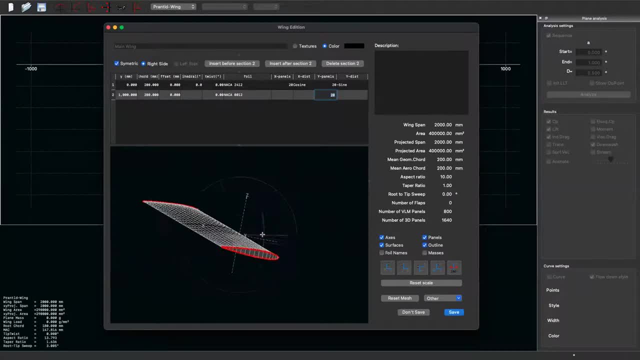 right. That's essentially what XFLR5 does, right, Just like how you use the loft command right. So you know, now we have a wing, right Now. let's, actually, you know, let's, let's do the. 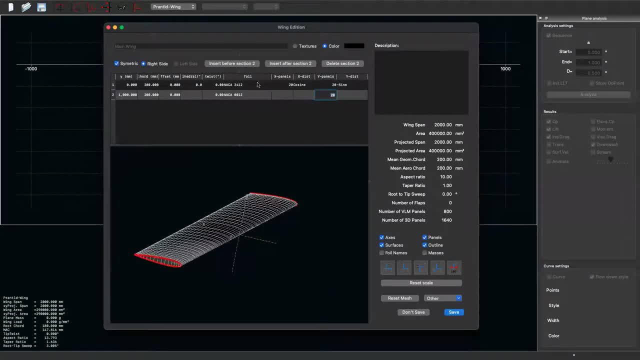 simulation and see how this looks like, before we come back here and change the twist and all that. all right, Now we want to make sure the baseline works right Before you add, before you add like any crazy you know shape or in any high twist. all right, Now let's. 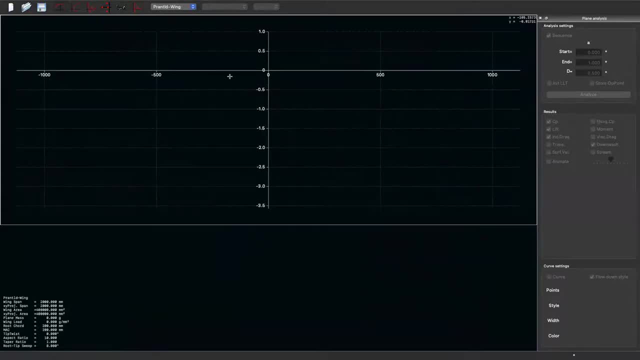 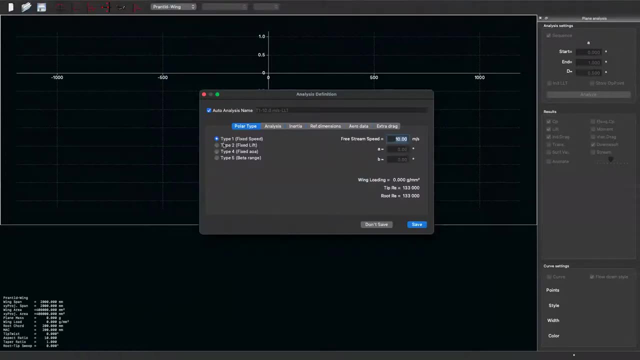 I'm going to click save here right Now. you know, you see nothing because we haven't performed an analysis. right, Let's go to analysis, define an analysis. Again, you have like multiple types of analysis you can do. but you know, we just we're just. 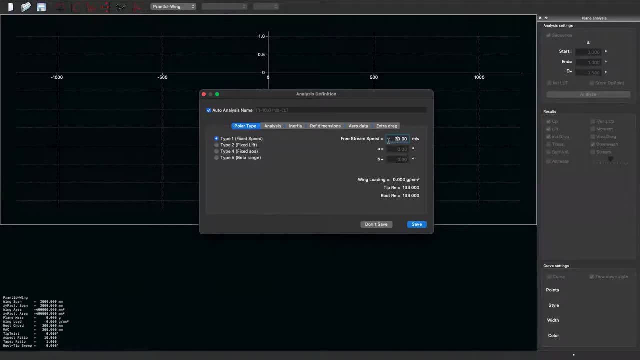 going to use the fixed speed. I'm going to use like 30 meters per second. We put the wing at 30 meters per second. Now, if we click analysis here, there are multiple types of analysis. right, You know, the popular ones are the lifting line theory and then the 3D panels. right, Let's start with the 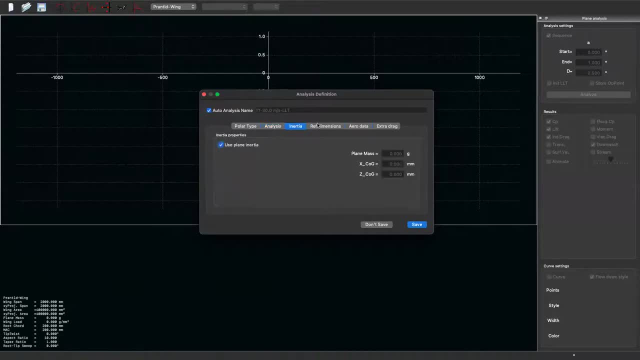 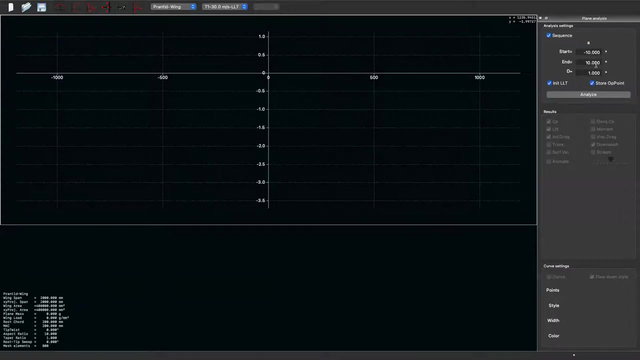 lifting line theory analysis. You know you can change the inertia and if you can change all of this if you want, but I'm going to leave it as such. I'm going to use the LLT lifting line theory first. right Now, let's click save. You can see the plane analysis tab has activated. right Goes. 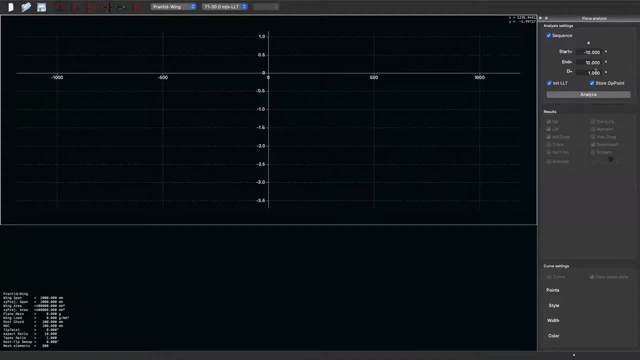 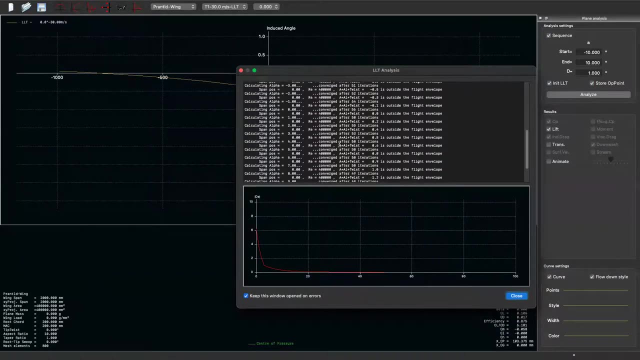 from negative 10 to positive 10 in increments of one degree, which is fine with me, So I'm going to click analyze right. So now you know it actually quickly performed the analysis. There are data points which are converged, but there are angles of attack which didn't converge. 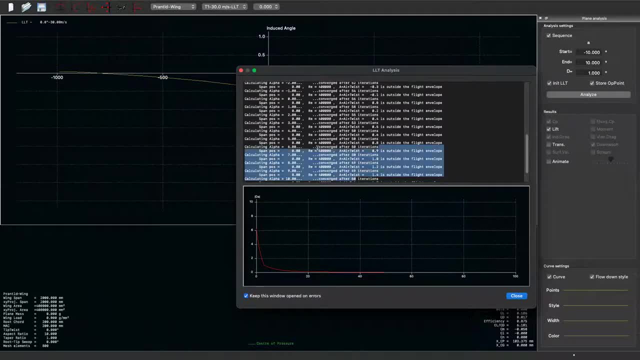 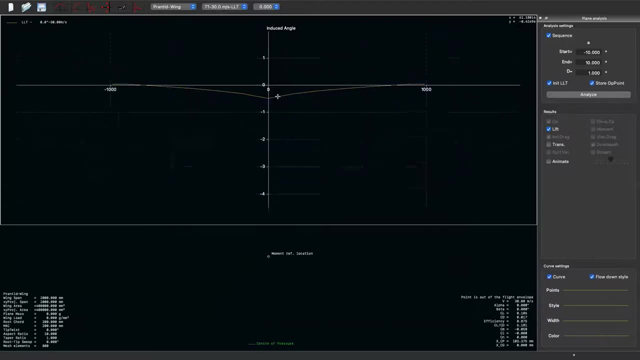 where you're not going to get any data. So just take a quick look at this. Make sure that you know this. you have majority of the angles of attack which are converged, All right, So we are done with that. Then, you know, close it. So you know, let's look at the first tab right here. This: 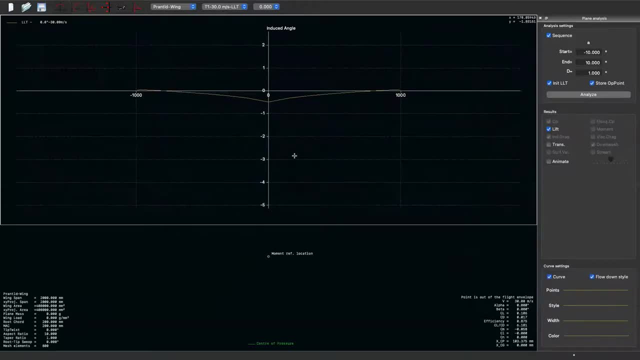 is essentially what you have right. This is. what you see here is plot of the induced angle of attack versus the span of the wing. All right, So what we're going to do is, you know, we're going to see how this induced angle changes the function of alpha right Now. look at that. That's that 10. 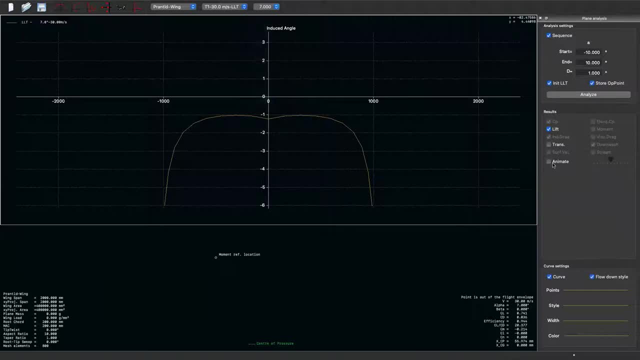 degrees. This is that. you know I can actually come here and click animate as well. You know you can see that as the angle of attack changes, what's really happening to my induced angle? right At negative degrees I'm creating like an induced angle and positive. 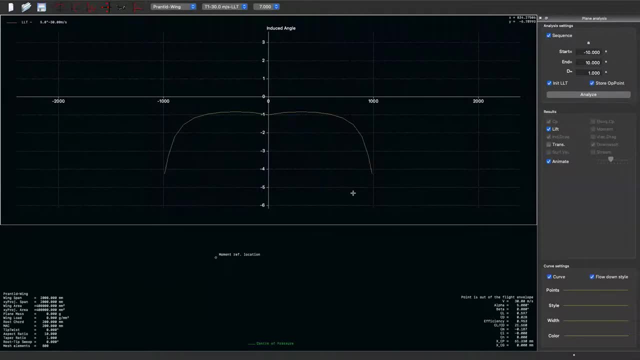 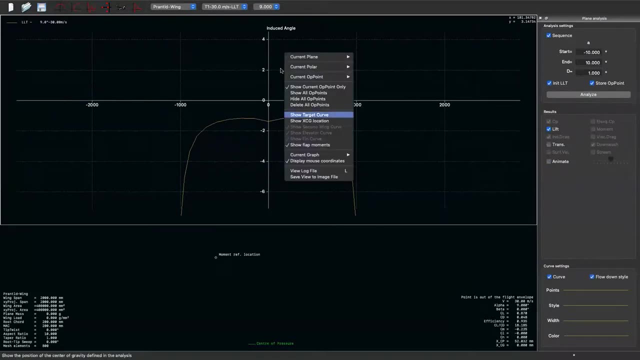 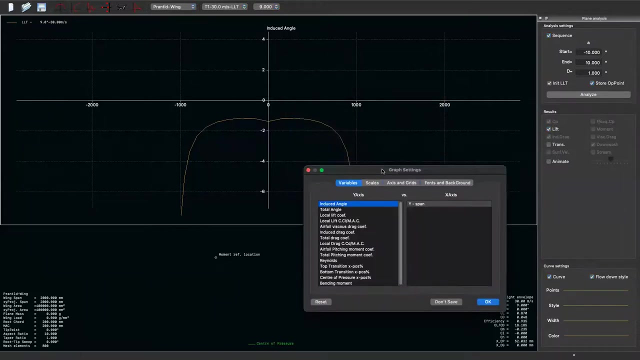 I'm creating like a negative induced angle, right, So that's great, You know. if you want to see other variables, you know, just go right click anywhere on this graph, do the current like graph right here. then you can actually define graph settings, right, So you can see here you're. 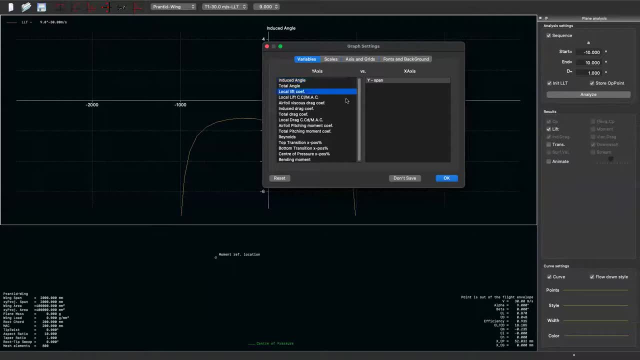 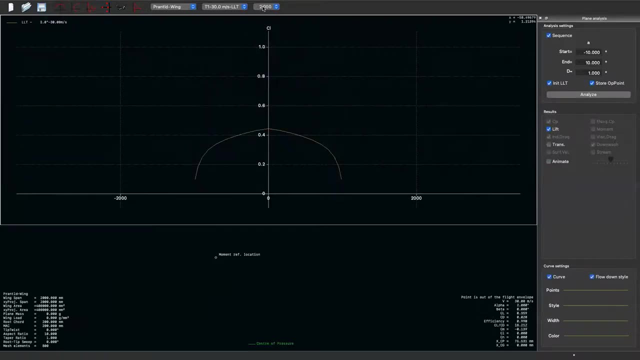 plotting induced angle versus Y. but you can also plot like lift coefficient. So you can see how the lift distribution looks like in here right At multiple angles of attack. So you can see here at multiple angles of attack right, Which is again pretty cool right Now if you want to. 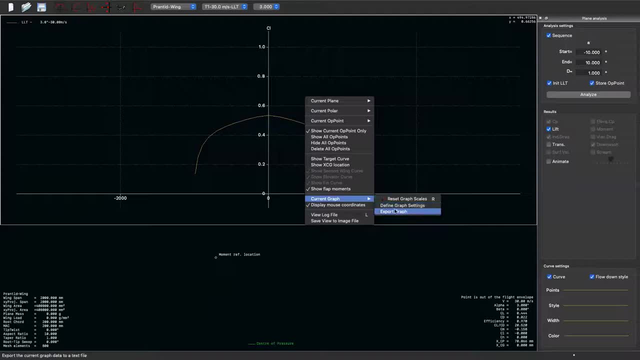 export this graph to be plotted in MATLAB or Excel. just do the export graph. you know it will actually export all of these. right, That's a tx. I think it may export as a csv file, but you know you can upload, you can open tcsv file in Excel or MATLAB, all right. So this is. 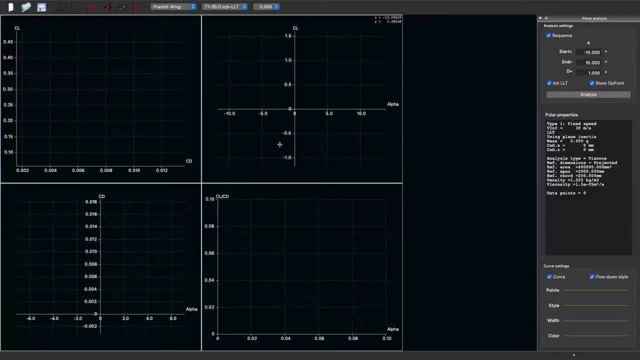 pretty great. Now if you, if we actually go here, you know, you don't see, you know any graph of a CL with a cd with alpha and anything for the lifting line theory, you know, I think it's predominantly because the LLT really, you know, it's all about getting the 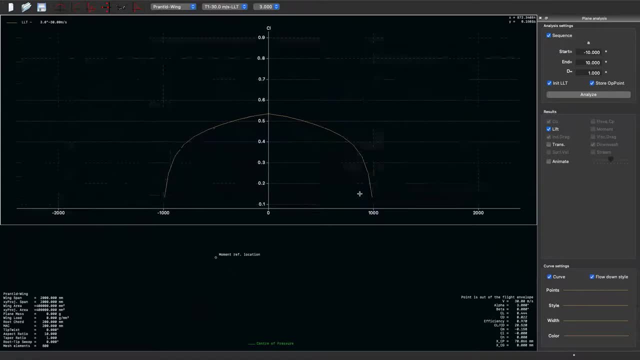 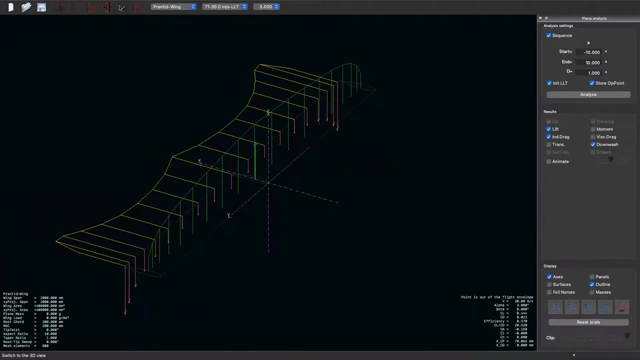 distribution for a given plan form, right? So you know, that's what. that's what you see here. However, you know, if you click this airplane icon right here, this airplane icon, you would actually get a distribution. So let me uncheck this, right? You know now you don't see anything in. 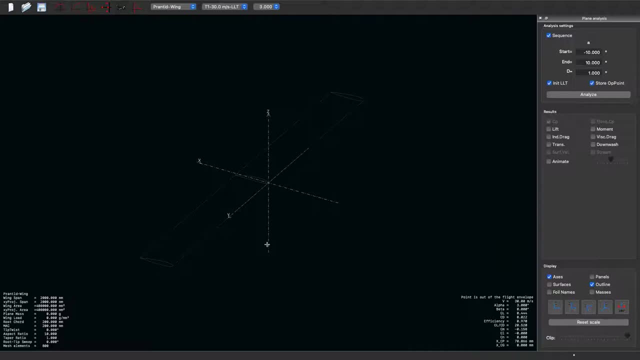 because you haven't you know the airplane color that we specified was black, right? So what I'm going to do is, you know, click panels. Now you can actually see the airplane right And you can click surfaces right. 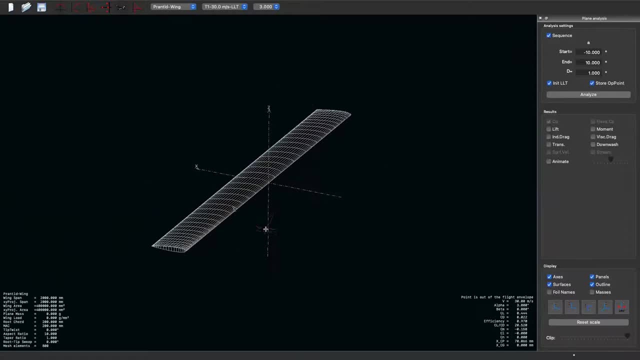 Now, this is the wing that we modeled. right Now, what I can do is actually come here and click lift right, But click lift. I can actually see the lift distribution on the wing And the cool thing is, I can animate it. 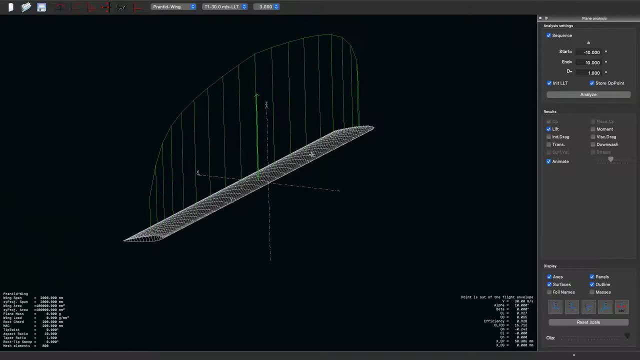 and I can see how the lift actually changes as a function of angle of attack. right, Which is pretty cool. You can see the wing changing the alpha as well. right, If I want to look at the induced drag. right, You know, I click this induced drag. 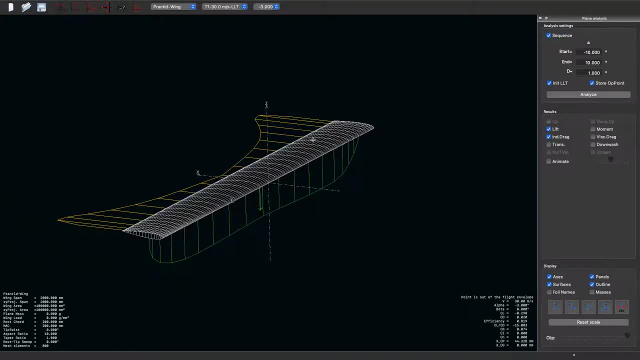 I can see the induced drag profile. right Now, the induced drag is higher at the wingtip because of the formation of the wingtip vertices. right, That's exactly what you expect And as you change the angle of attack, right. 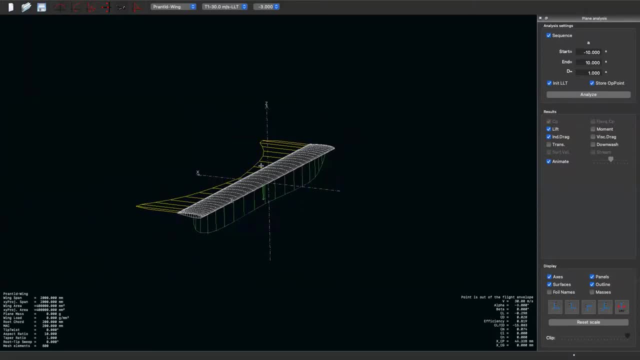 you're creating more and more lift. So you know you will have a stronger vertices which will, you know, have a higher, like an induced angle. you know induced drag at the tip right. So that's essentially what you're seeing. 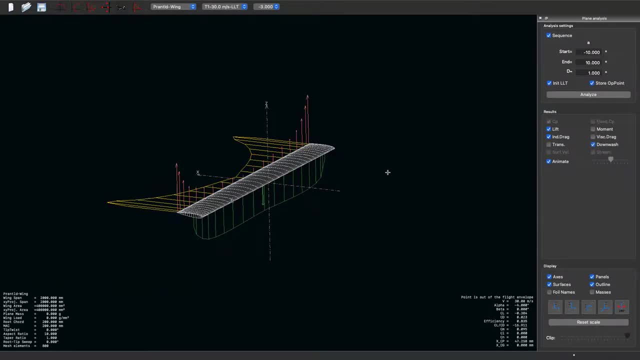 What you can also do is actually click downwash right. If you click the downwash, you know you can see that the downwash profile in the red curve right, Which is again pretty cool At positive angles of attack, as you can see right. 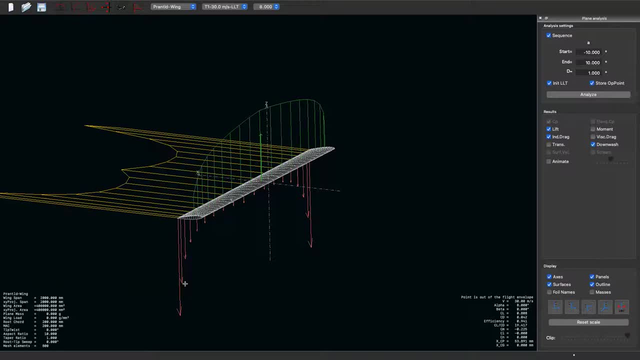 because of the vortices you have a huge downwash near the wingtip and it reduces as you move towards the root of the wing right Again, due to the span changing right, you know the distance from the vortex changes. 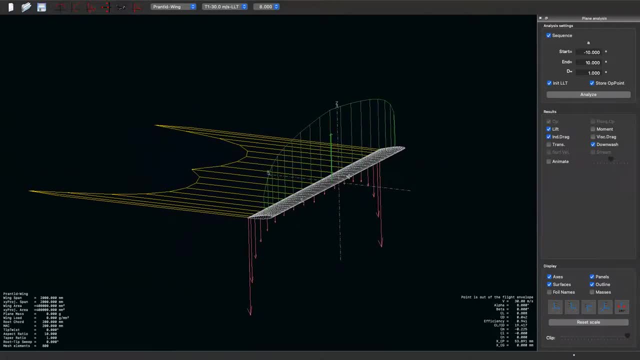 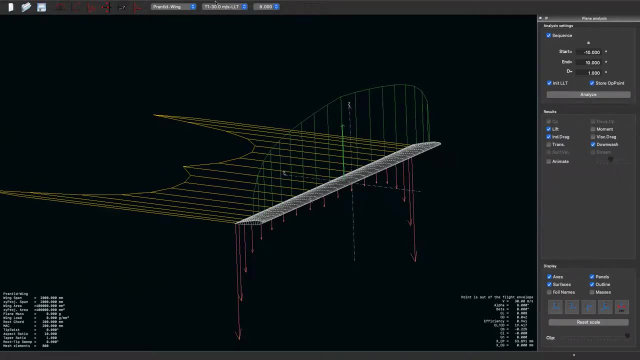 they'll have less influence. So you know you have less downwash at the tip, right. So again, it's pretty cool that you were able to see this and you can plot from different angles of attack in any angles of attack that you want, right. 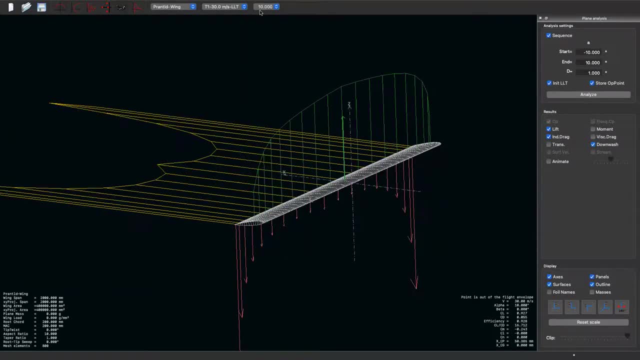 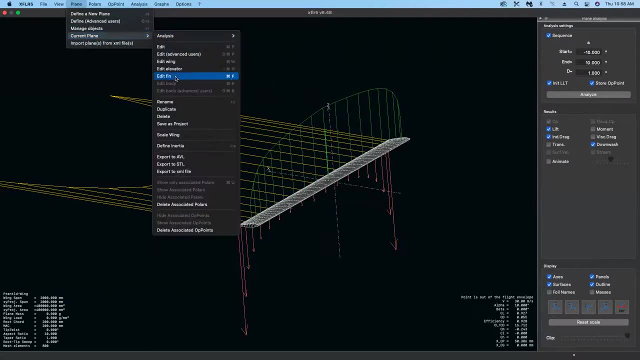 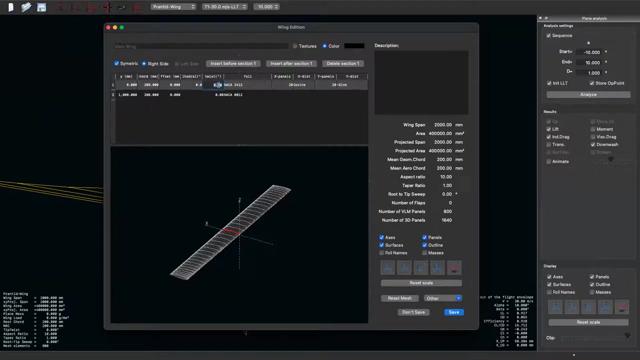 So again, this actually works right. So now what we can do is go back to our plane. right Now we can actually add, start adding twists. all right, So we go back to plane Again. I'm going to put my root chord at about, like maybe eight degrees. 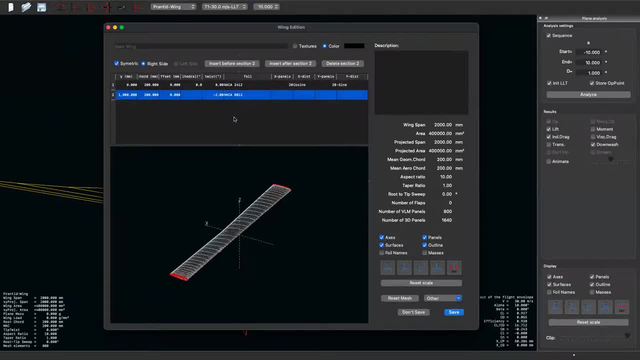 and then my tip chord as about negative two degrees right Now, this is just a distribution. Again, you know this is just to get that high jump, but this is just a geometric distribution that they're using on panel D aircraft. all right, 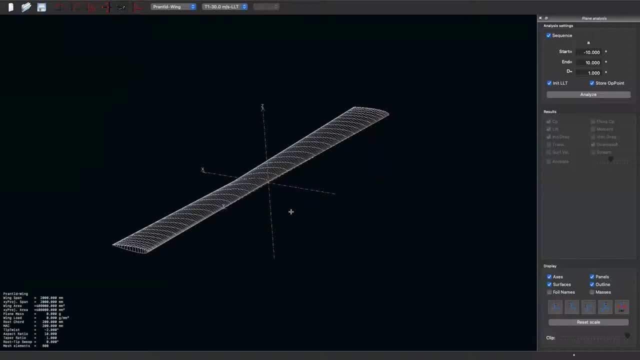 So let's go click save. Okay, you're not going to see any curves here because you haven't performed the analysis. However, you know, if you look at the side view, you know you can actually see the twist that you included, right? 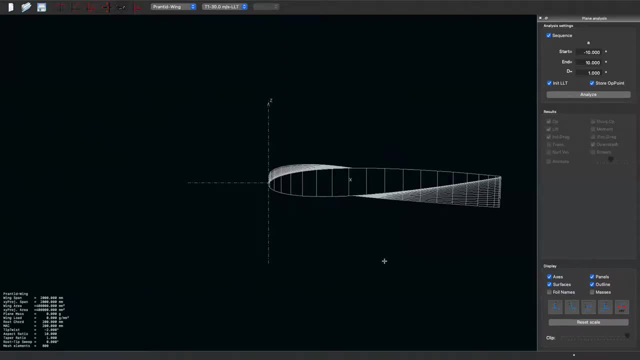 The root is at a high angles of attack when compared to the wing tip, which is exactly what they have on panel D right Now. if you want the exact specifications of panel D, you can go search online. you can have it programmed in the. 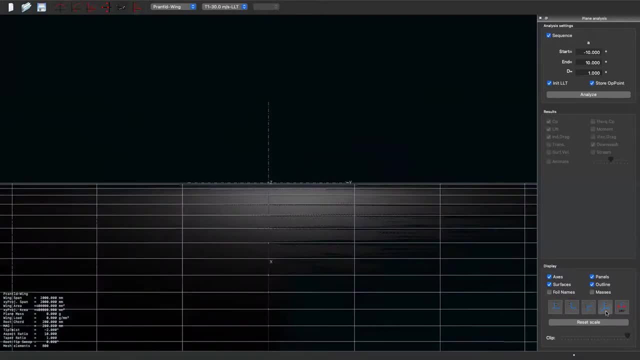 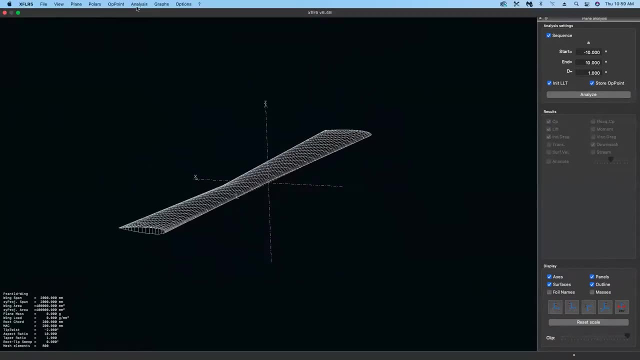 have it modeled in, you know, in this, in the XFLR five. But for now we're just going to go with this in an arbitrary twist. distribution. right Now let's go back here again, go to analysis. fixed wing: 13 meters per second. 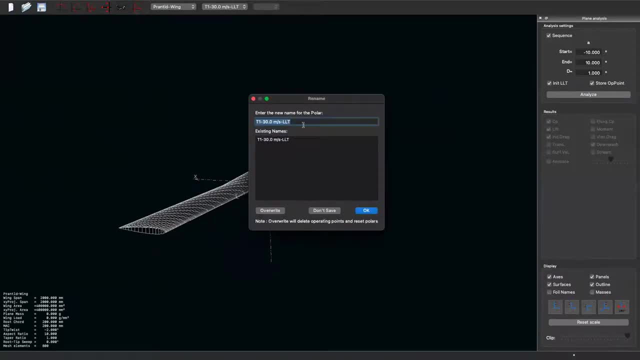 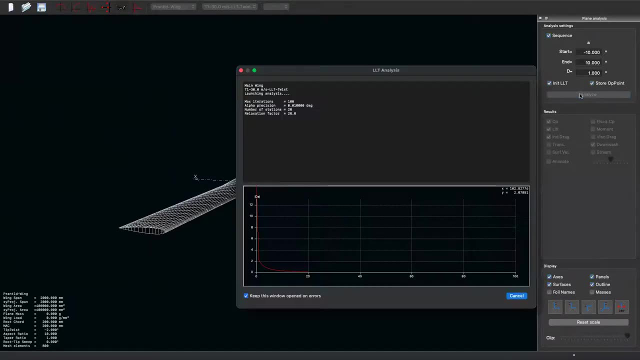 LLT. that's all right. You know. click save. You know I'm going to create another file called Twist. click OK. now it's performed, the analysis. Now you can see. you know I've made this also. 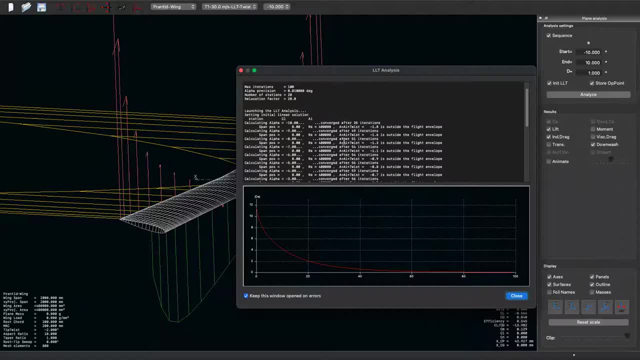 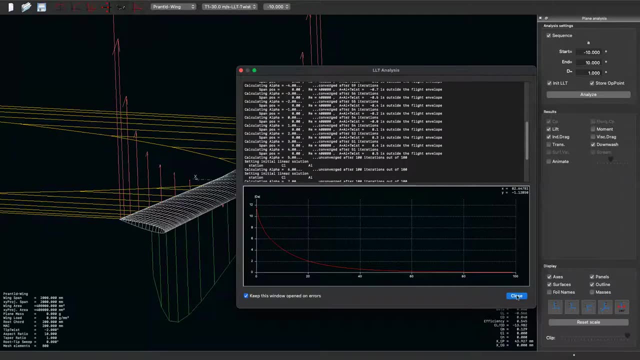 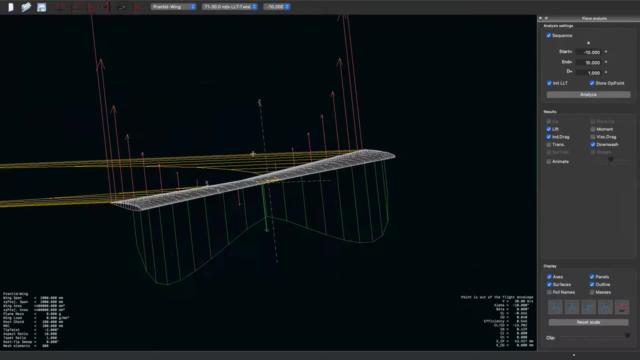 see here again that some of the values are not not converged, which is fine. as long as you have more angles of attack which are converged, you'll still be able to see the data. all right, so now you can actually see the variations in um. you know the, the, the lift distribution, the induced 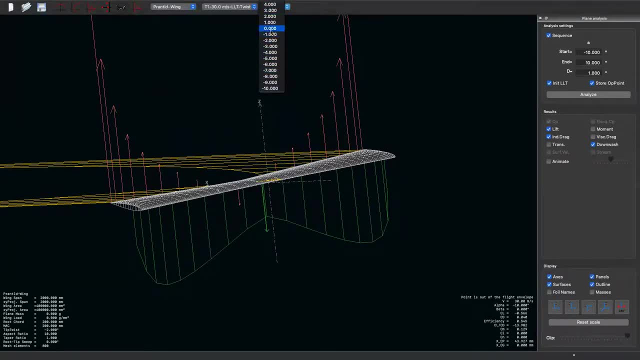 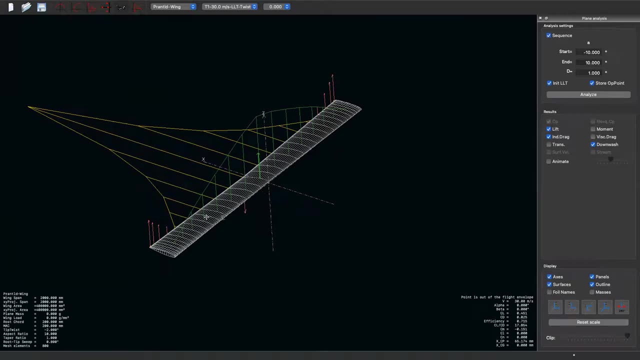 drag and downwash. let me put at zero degrees. um, so i have zero degrees right here, right now. you can see that when compared to a no twist uh distribution, the, the lift distribution looks a little different like. it looks a little bit more like a bell-shaped lift distribution than 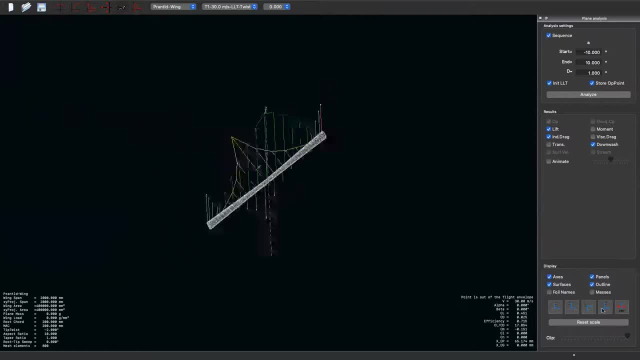 anything else. um, one other thing also to note is that that we want is- uh, let me go back to the back view here. right now, if you look at the downwash distribution, what you see here are arrows pointing up right, so that's actually an upwash. right now, you can actually get the upwash. 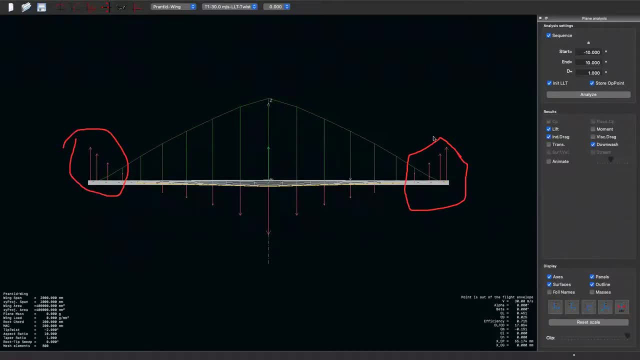 distribution. now this upwash is actually is responsible for induced thrust um, which actually gives you a proverse yaw um right, which makes the airplane yaw in the right direction, uh, as in roll right. this is essentially what the panel d does, and this is exactly what we wanted to see. 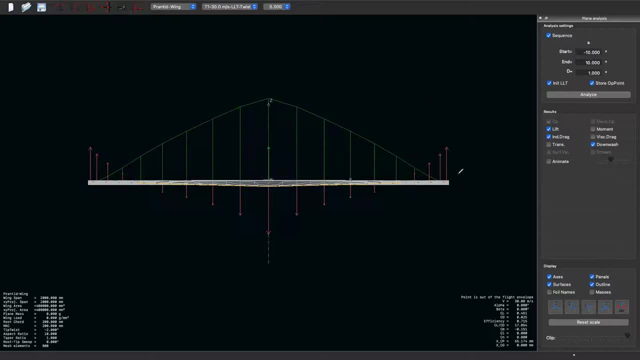 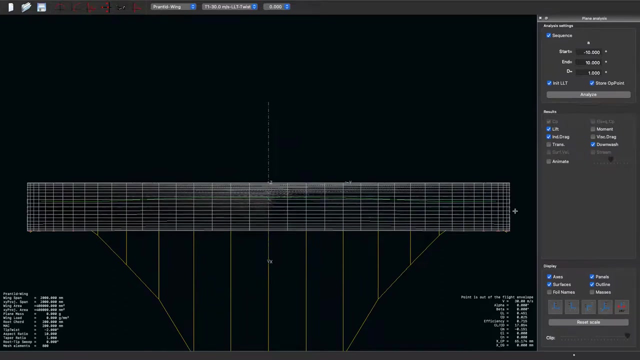 right. so um, again, you can. you can see that it's, uh, the positive upwash direction, which is actually pretty cool now. now you know you can look that. look at that in the induced um angle as well. so there is a small portion of the induced drag which goes. 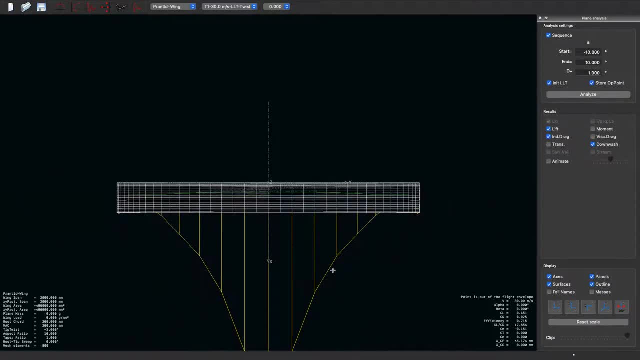 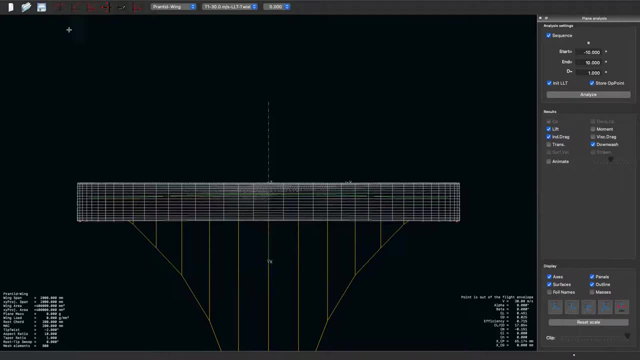 positive, which tells you there is an induced uh positive, induced uh drag, which is actually the induced thrust. all right, so um, you can actually see that pretty clearly. you know, in this plot, right here. if you click on this, you know you can see that cl versus the span distribution. 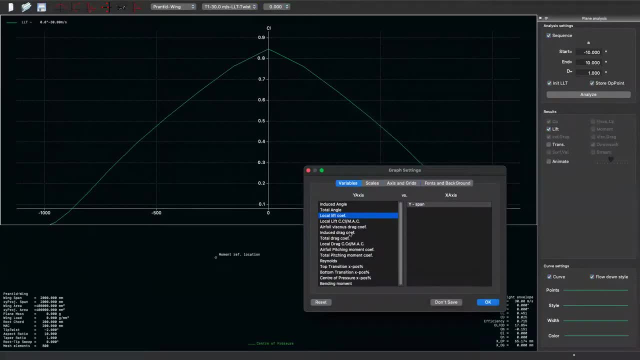 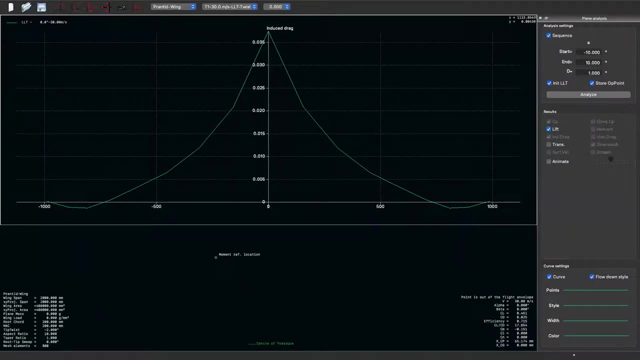 um, and again i can go back and change. now i want to look at my induced drag coefficient. click on it. Okay, so you can actually see that there is a portion along the wingtip where you have a negative, like induced drag. you know, negative drag is simply thrust right. 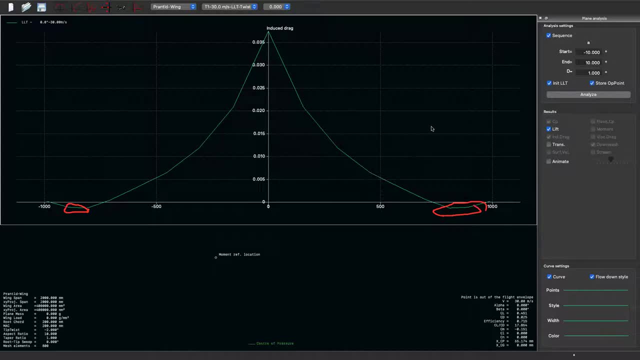 So negative induced drag. so that means that's a positive induced thrust which makes the airplane yaw in the right direction of the roll right. This is again pretty cool how it works right And you can do several analysis, you know. look at multiple angles of attack, right. 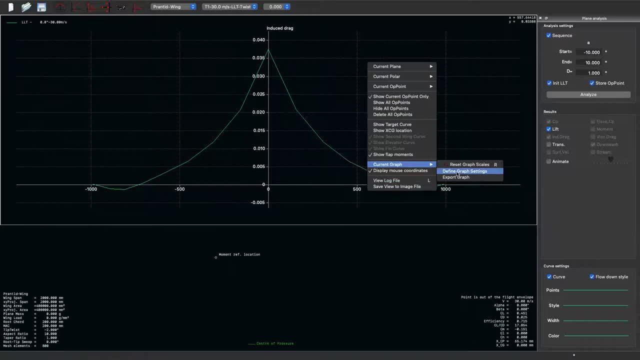 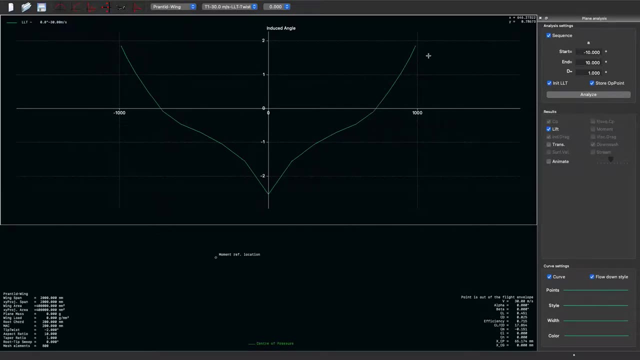 You know, I would urge you to, like you know, look at multiple parameters so that you have a good understanding of what's going on. right, So you can look at the induced angle. right, You know, you can see the high positive induced angle at the tip right. 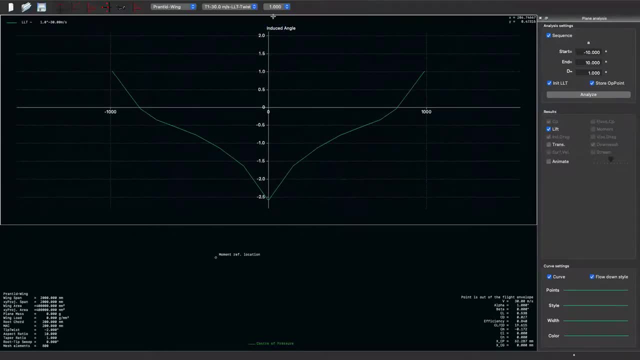 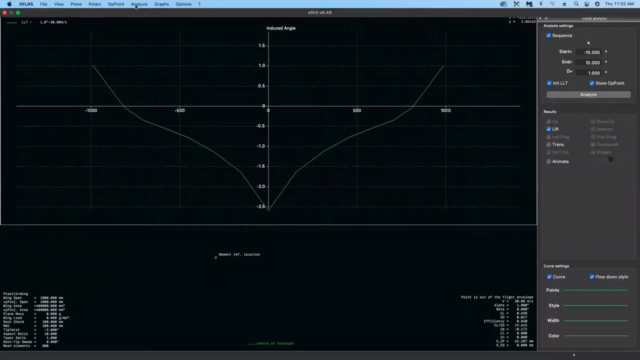 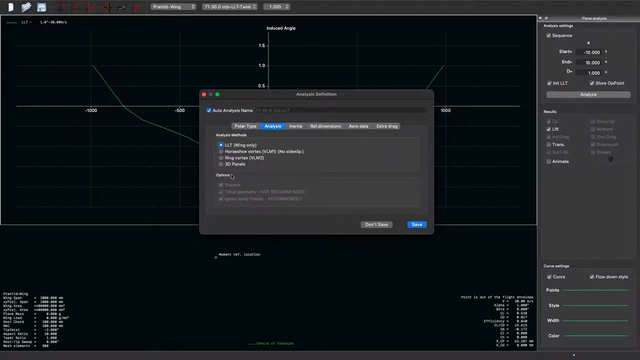 Now that changes as a function of angle of attack, but you know, you get this induced thrust at low angles of attack, which is essentially how you cruise right, So this is pretty cool. Now, before we end this video, I do want to point you guys towards a- you know, the different analysis tab called 3D panels, because this will allow you to get the CP distribution on the wing all right. 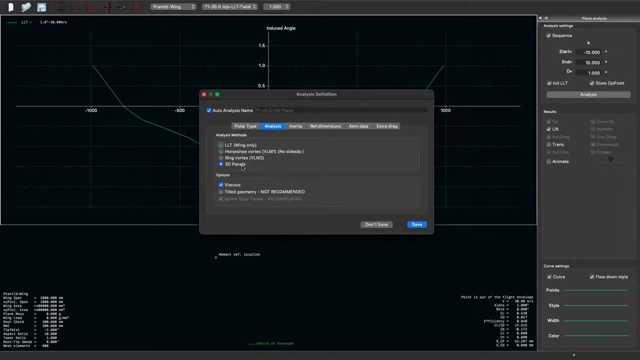 Now let's go to check and let's click the 3D panels. You know, let's uncheck the viscous because viscous simulation is a lot messier and probably you're not going to get a good comparison Convergence right. 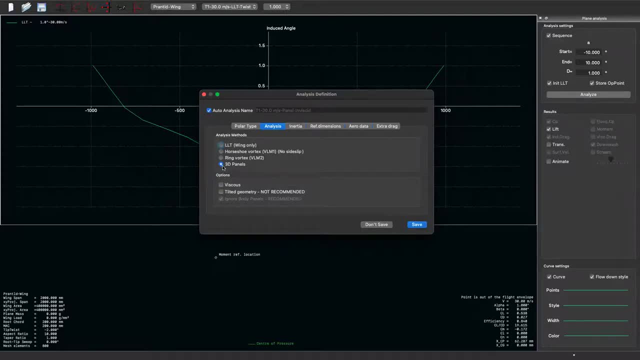 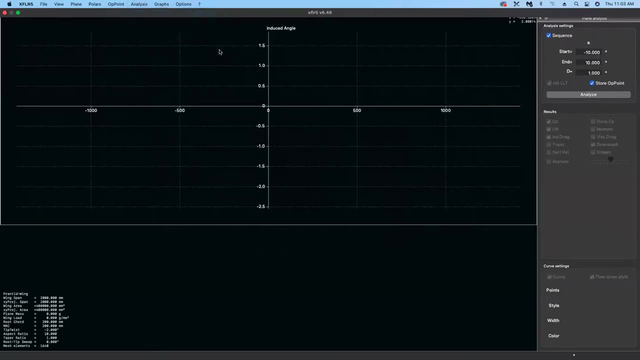 So let's stick with the inviscid analysis. It's, you know, click 3D panels, uncheck viscous and click save, All right. Now again, we need to define the analysis because you know, oh you know, we just we just defined the 3D panels right. 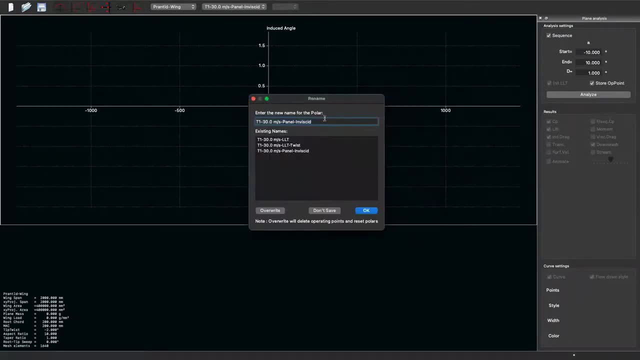 Uncheck viscous. you know that's good, So let's let's you know. yeah, this is the panel inviscid, which is which is which is what we need. Click okay, All right, So let's. 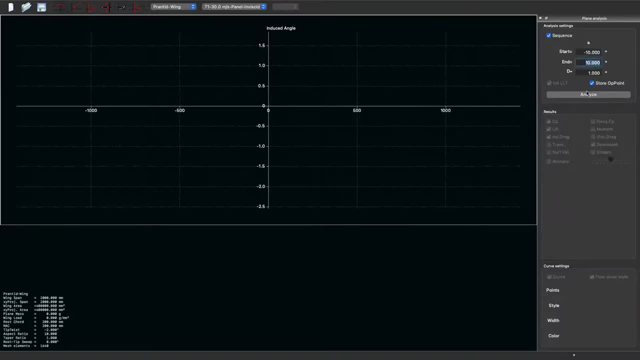 Once again simulate from negative 10 to 10 and increments of one Click analyze. right Now. this may take some time, right? So the more number of panels you have, the higher the computational time will be, All right. 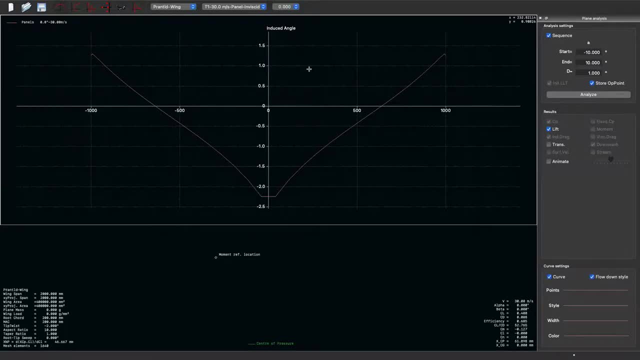 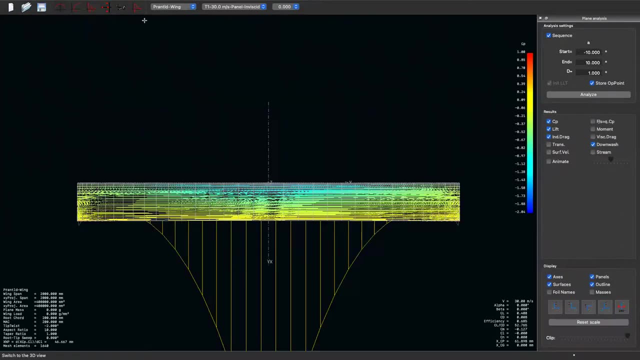 So you can see that. you know, in this case, in 3D panels, most of the angles of attack are converged right, Which is again pretty cool. However, one really interesting aspect of the 3D panel analysis is that it will: 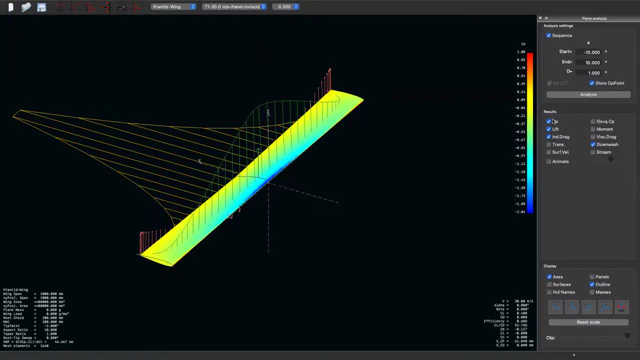 Give you a CP distribution. on the wing right I'm going to uncheck the lift in this triangle and all that. Look at that. That's my CP distribution. Now you all should know by now what a CP is. coefficient of pressure is right. 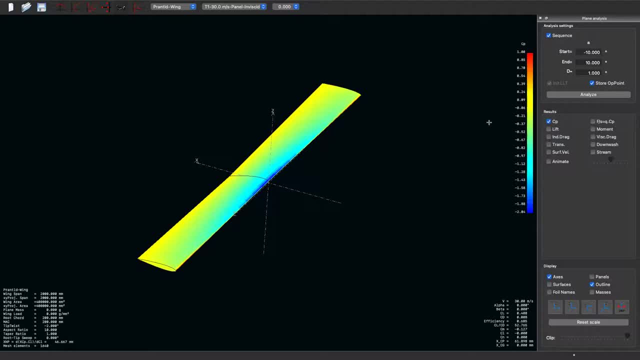 It tells you how the velocity is actually changing across the wing when compared to the free stream, And that by giving you an idea of what the pressure is doing right Now. if I animate it right, you know you can see what the what the pressure distribution looks like. 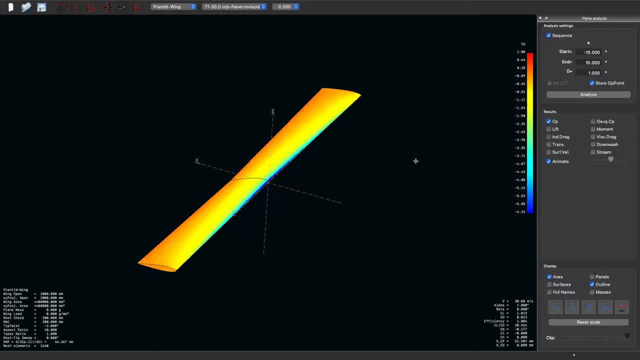 Um, across Your wingspan right As you change the angle of attack, which again is actually pretty cool. Um, right now you can superimpose the lift distribution on top. Um, you can have the induced drag distribution. You can see that there's a certain 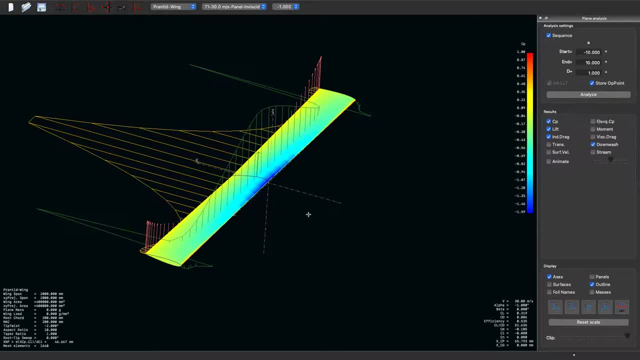 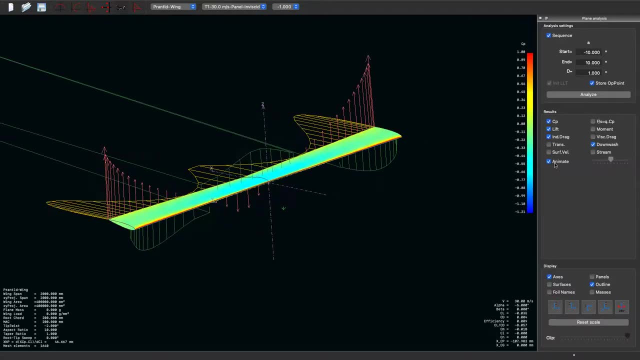 Thrust induced stress you're getting and you can actually have the downwash as well. Now you can actually see the upwash along the winter right. So if you animate it, you can see how that changes as a function of span and you know, make sure that you have, uh, the good conclusion. 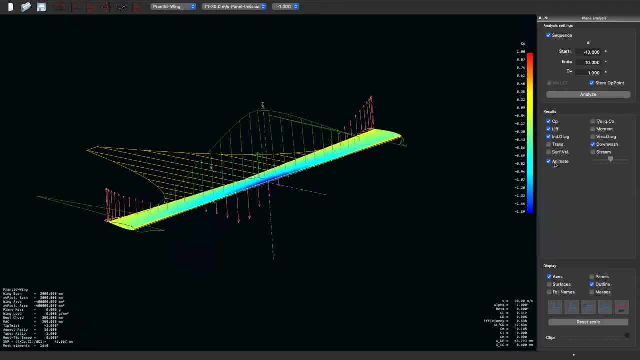 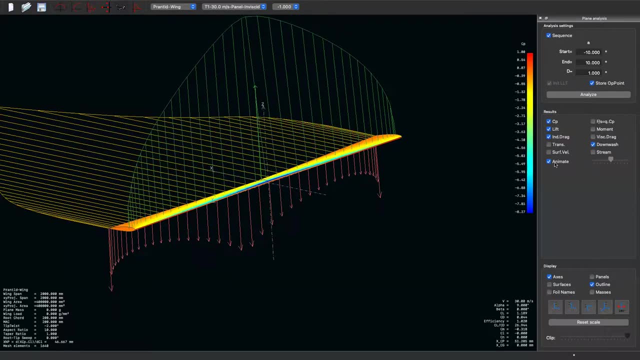 Connection, uh, you know, between what's going on, the downwash, the lift and the induced drag, right? So this is add in fact pretty cool. uh, you know to see, right, And you know if I have multiple angles of attack. 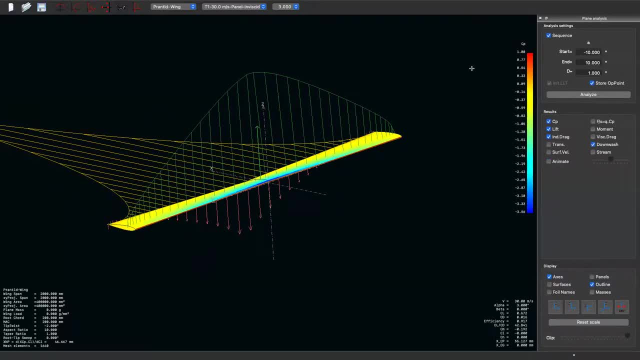 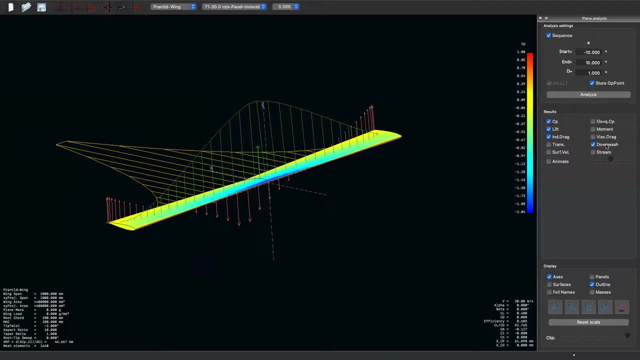 So another cool thing that you can also do is: you know, I'm going to put the airplane or the wing at zero degrees. right, You have the induced thrust, uh, you see the upwash, uh, on the wingtip. 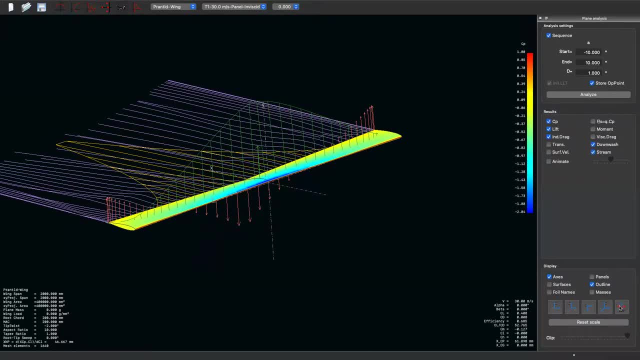 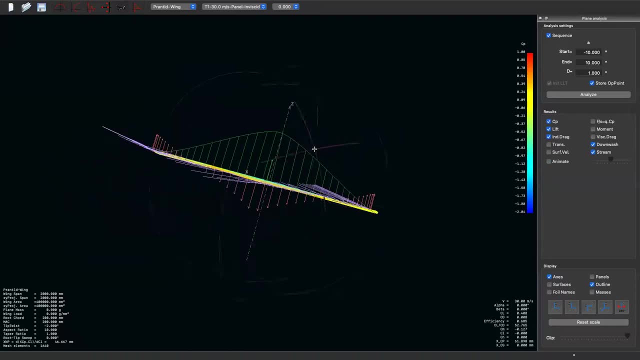 Now, actually I can, I'm going to click stream So that will allow me to see the flow. Um lines behind the air for behind the wing Right. So again, um, let me look at the back view right here. 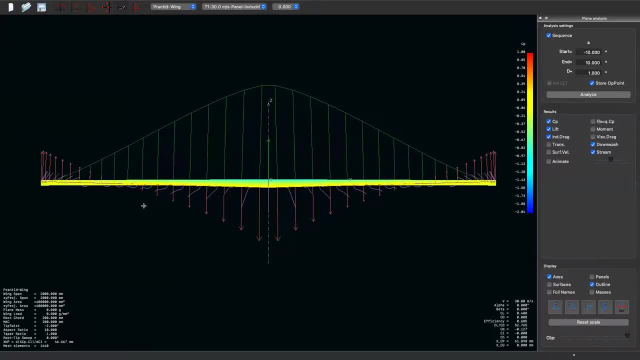 So you can see that. you know the there are roll up of small vortices. Let me uncheck: uh, all of these right, Um, right now, because of the down upwash, you can see the vortices are rolling up. 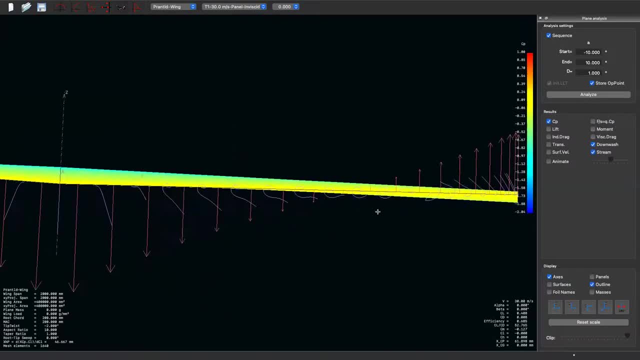 You can see the, the, the curvature right here. right You can see the stream. it's curving right. So essentially, this shows you The wing vortex instead of the wingtip vortex that you have on a regular airplane, right? 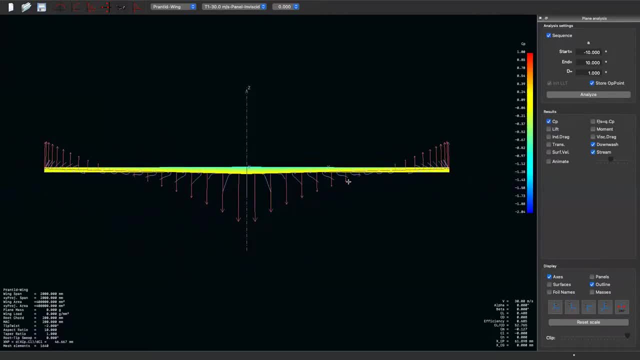 So in this configuration you don't have a wingtip vortex. You have a wing vortex. right now, as you keep increasing the angle of attack, that wing vortex is going to move towards the tip right here, Right, Um. again, it's pretty cool that you you know that that in Prandtl-D, uh at, uh, at low angles of attack, you don't have a wingtip vortex. 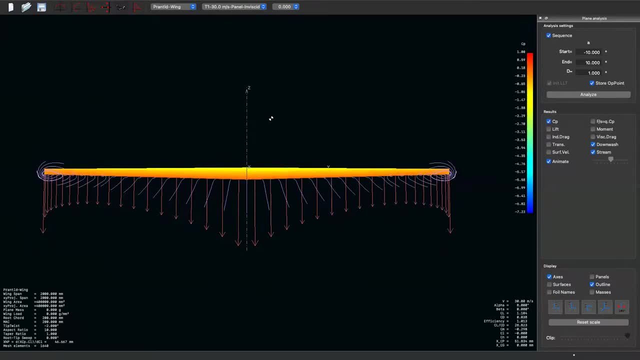 You have a wing vortex. You have a wing vortex right, Which is uh, which is again uh, you know, really cool, Um, um, you know, let me show you the um, the platform view as well, or the isometric view. 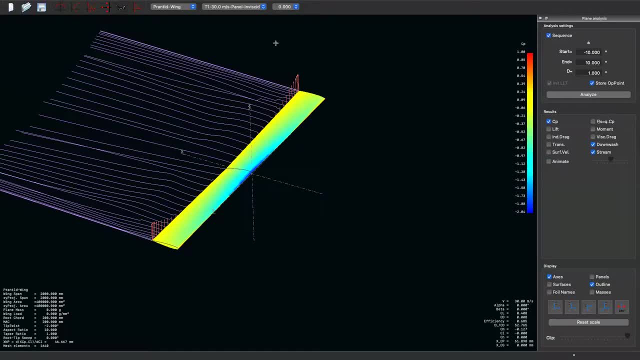 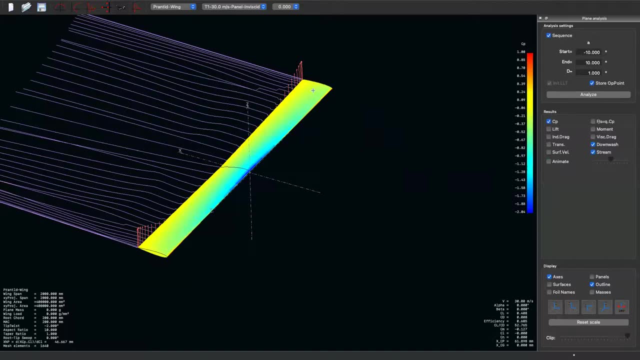 So again, you don't see that, uh, that wingtip vortex, even though we look at the lift CL, the airplane is, the wing is producing a CL of 0.4 and you don't see the vortex right. And you see the wing vortex in here. 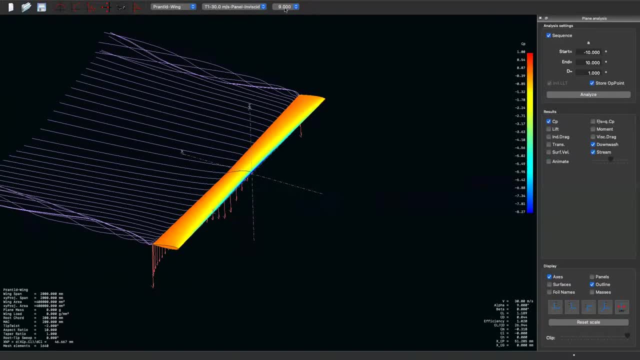 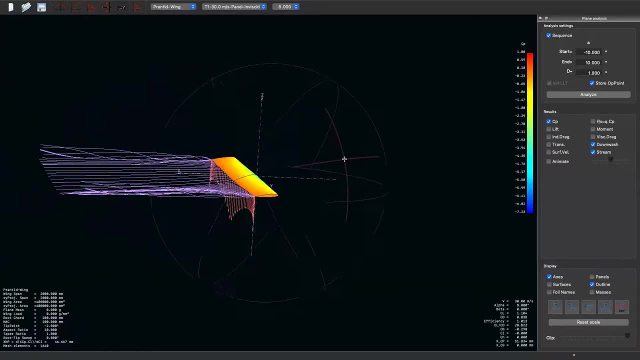 Um, but as you keep increasing the angle of attack, now you see it clear. You see the rotation uh of the, of the vortex Right, Um, which is again the really cool um uh aspect. you know, it's really cool that you can actually see this. 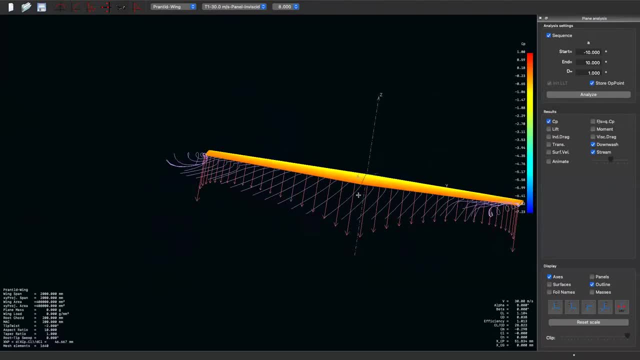 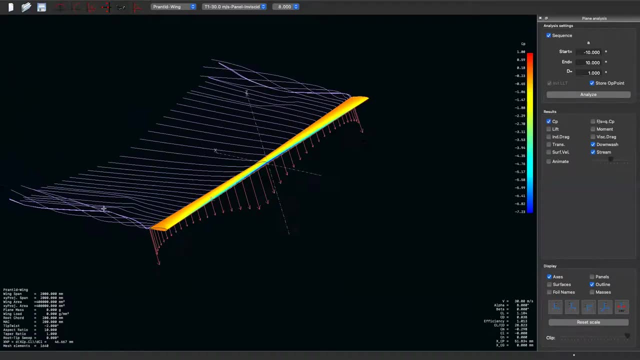 You can see the rollup of the vortices and make strong connections between the different aspects of finite wing. right, You know, finite wing is a lot more interesting than airfoil because you have a distribution and you can do a lot of cool things right now. 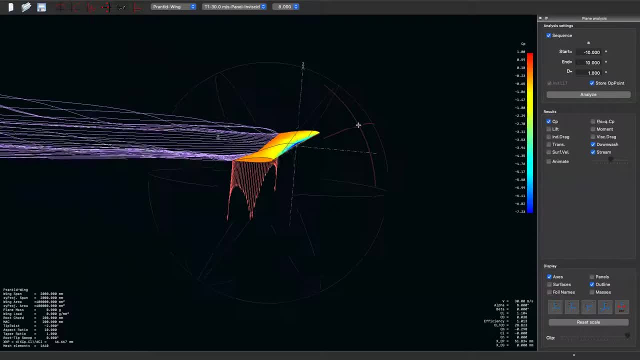 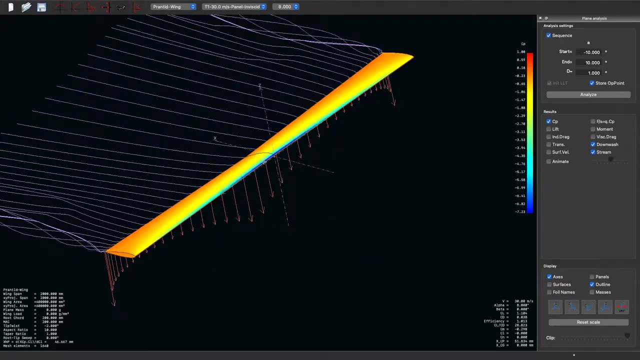 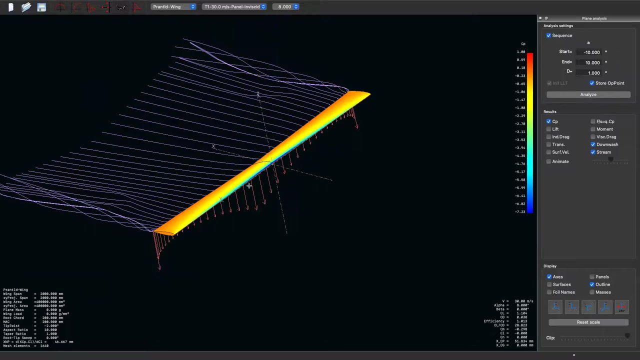 We have different airfoils, We have different wrist distributions, and all of that will give you a different performance. And that kind of comes back to the art of wing design. right, You can essentially get any shape you want: um, uh on any, um, any, uh, uh, Force distribution, CL distribution you want on top of a wing, by changing the twist. 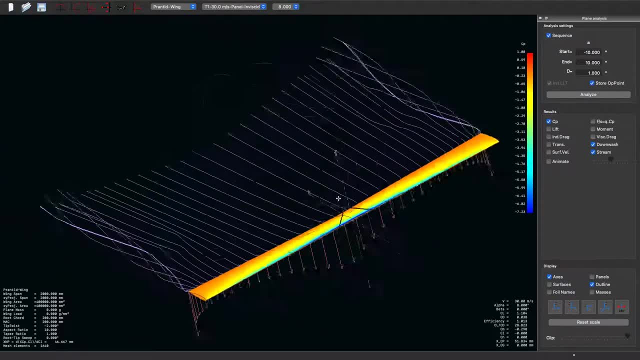 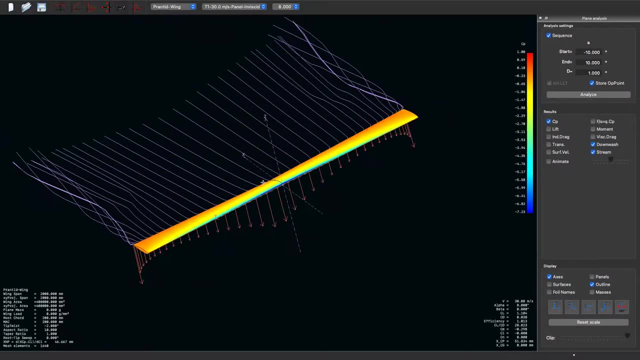 Now this is all inviscid, right? I mean, if you turn on viscous analysis, uh, there may be some separations going on. you know, we didn't, we're not accounting for that, but uh, in, even from a pure understanding standpoint. 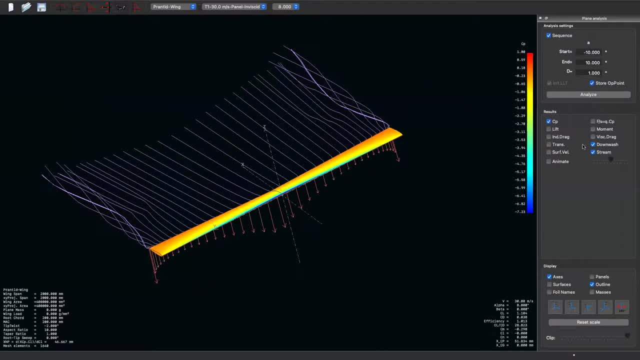 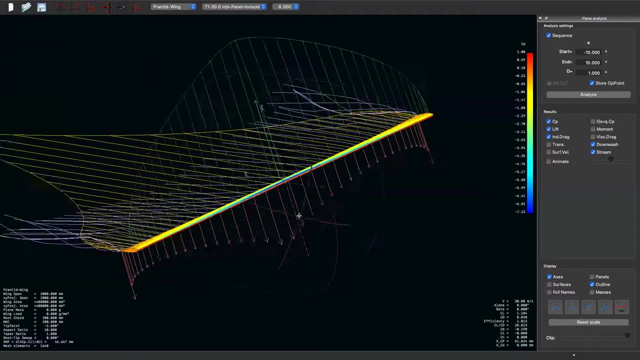 I think, I think this is a pretty good, pretty good tool for allowing you to visualize what's really happening and the relationship between all of these different uh parameters. Uh, that's that's very important in a, in a wing, um, in a finite wing. 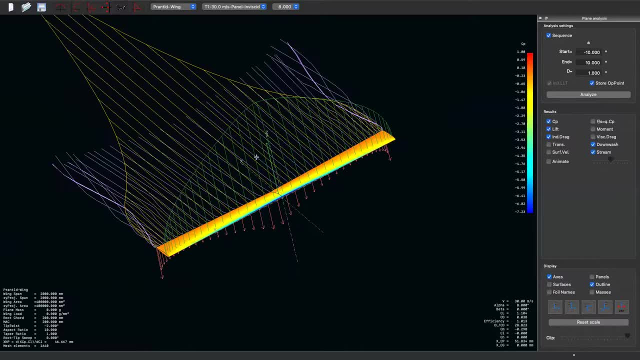 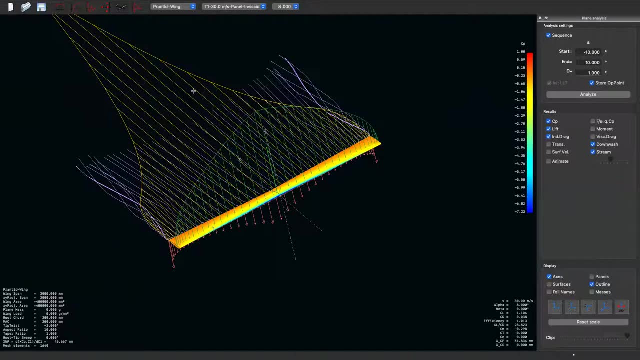 All right, Um hope you enjoy this video. Can? I hope this kind of gives you a good idea of what to do with XFLR5 and how you can simulate the wing uh model and, you know, extract parameters. Um right. 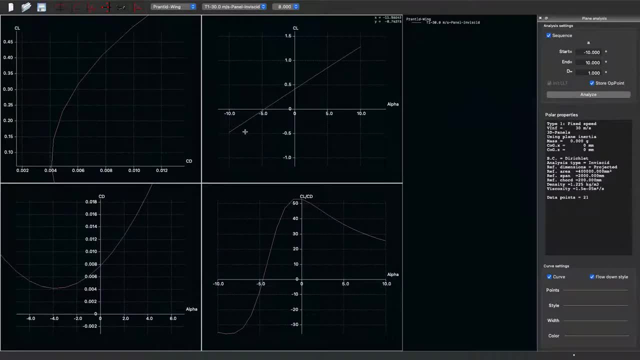 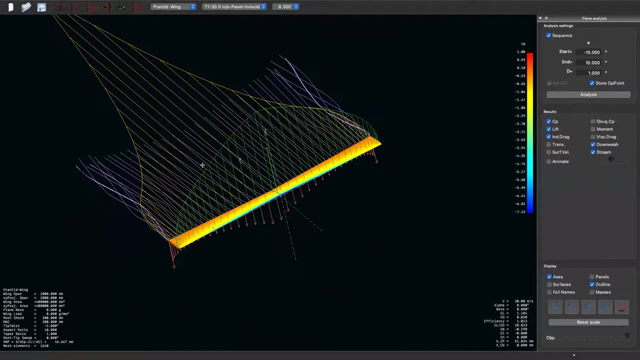 So, um, another thing before We leave is that you know when you the 3D panel analysis will also give you a nice uh, CL versus alpha curve, CD versus alpha curve and all that. So you know what the overall net CL and CD and everything is at a given angle of attack. 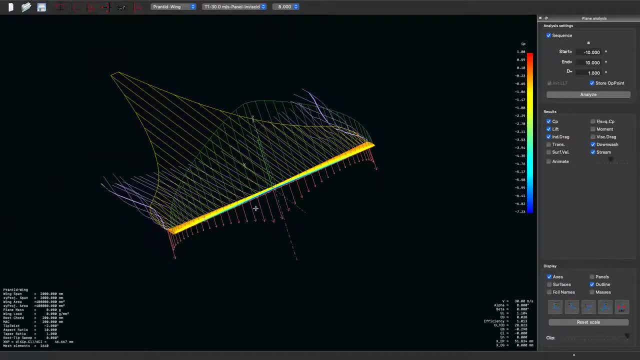 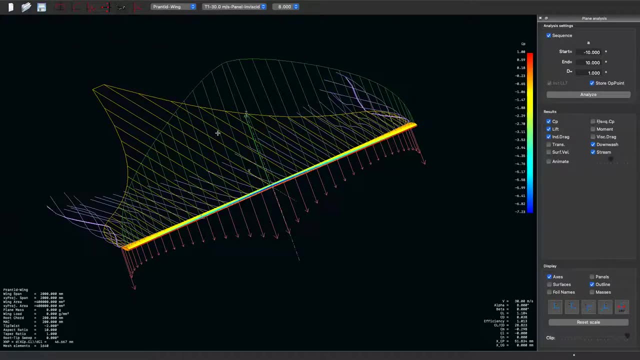 All right, So hope you enjoyed this video. Um, you know, uh, hope, uh, you use XFLR5 in your future and, uh, you know, understand the aerodynamics of finite wings. All right, Bye. 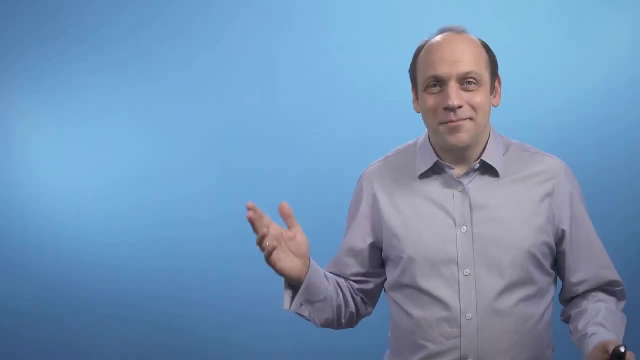 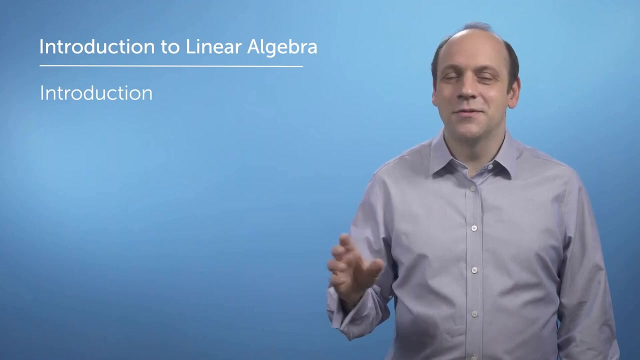 Hi there, I'm David Dye and I'm going to introduce you to this course on linear algebra. Later in the course, Dr Sam Cooper will take you through the last module and in his course on multivariate calculus I'll do a bit in return, But in this video I just want to take 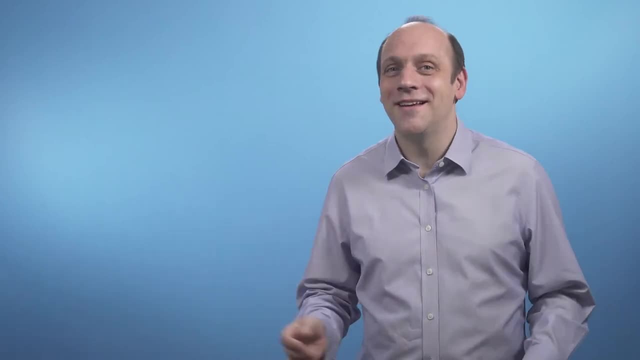 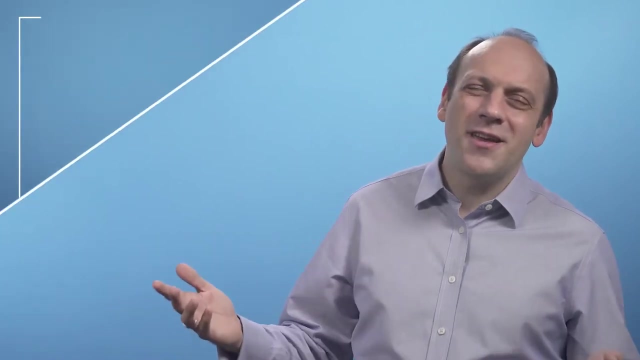 a moment to introduce the course and what we're trying to do here and to set the scene. The world is awash with huge amounts of data. Most of us living in cities generate huge amounts of data as we go about our lives moving around browsing our mobile phones. 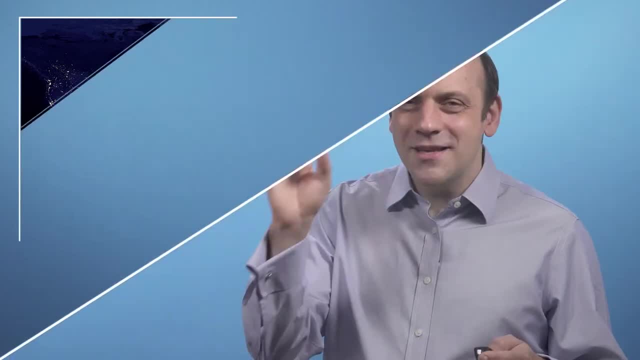 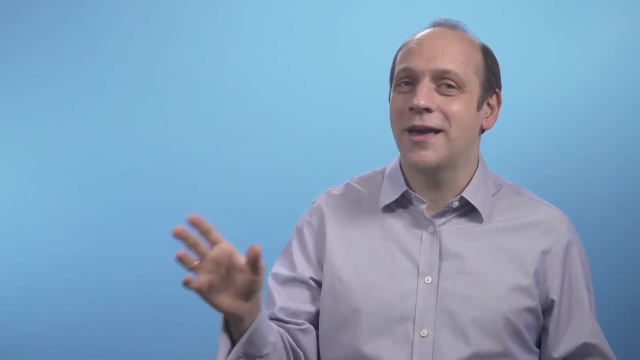 using transit networks and consuming energy. If we just think about energy alone for a moment, our society literally lights up our planet from space. We can see where the people and economic activity are from the light Zooming into Europe and London. here you can. 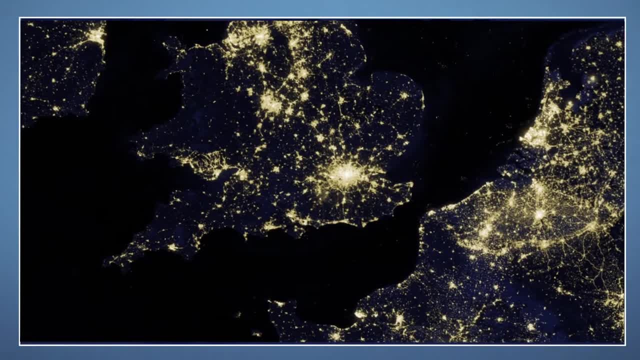 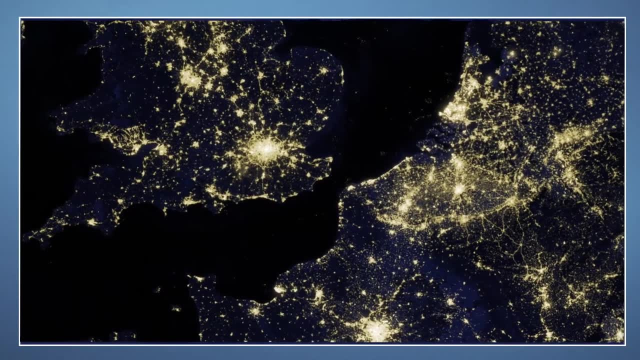 see how some of the world's great cities network together. This takes a huge amount of energy, and if we're going to figure out how we're going to generate and use energy more sensibly in the future, we're going to have to understand the data. 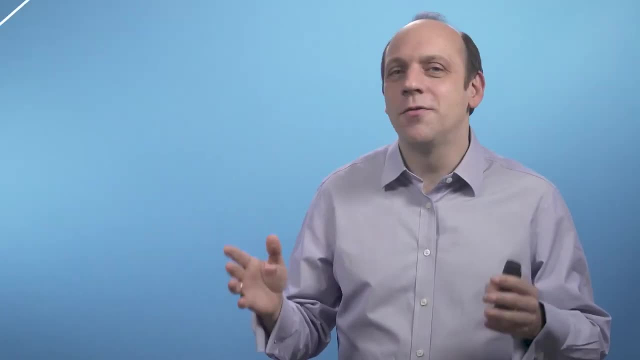 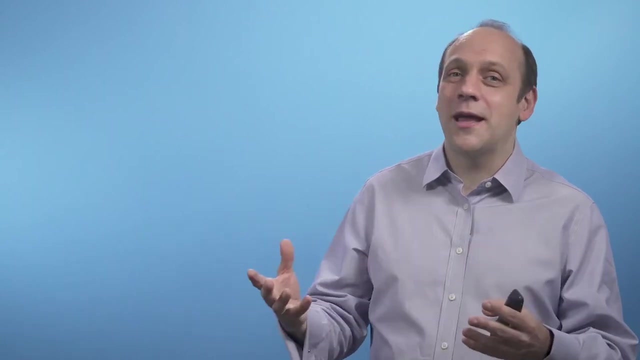 we have about energy much better. If we don't want to damage our health with NOx and particulates, and if we want to combat global warming, we're probably going to have to strongly cut back or even eliminate burning hydrocarbons as the leading approach to powering our society.